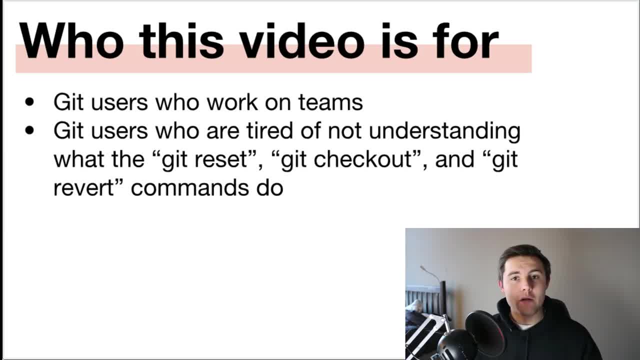 two videos, and that is the fact that we had no problems to deal with along the way. We pretty much assumed perfect conditions. We assumed that everyone on our team was working perfectly in tandem and there was no conflicts going on at any point with our repository. Now this is far from. 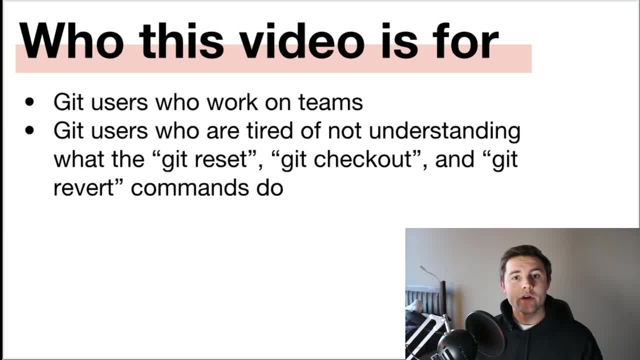 a realistic scenario And in real life. you're going to run into plenty of problems with the Git source control tool, And half the battle is knowing how to resolve those problems without having to pretty much reset the entire workflow Repository. So this video is going to be perfect for anyone who is either working on a team or 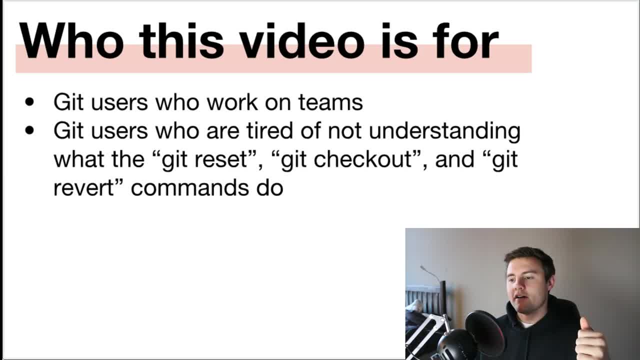 maybe you're like myself and you finally got tired of not understanding what the Git reset, the Git checkout and the Git revert commands do. So these three commands are all commands relating to kind of troubleshooting your repository and switching between branches in your repository And so 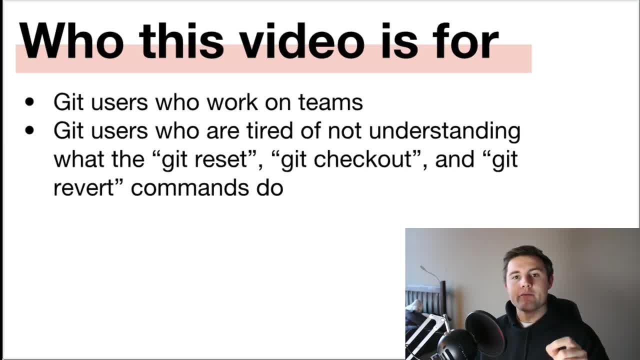 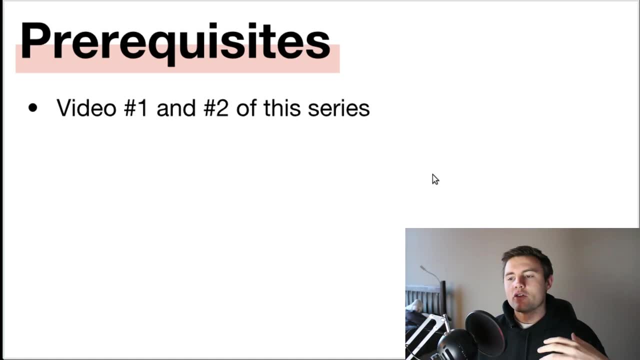 there we go, So you'll learn in this video a deep dive of those commands And you'll finally understand how do we actually resolve conflicts in our repository. Now this has two prerequisites. That would be video number one and number two, If you're already. 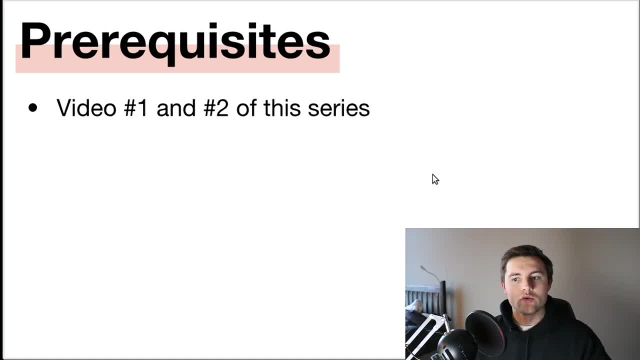 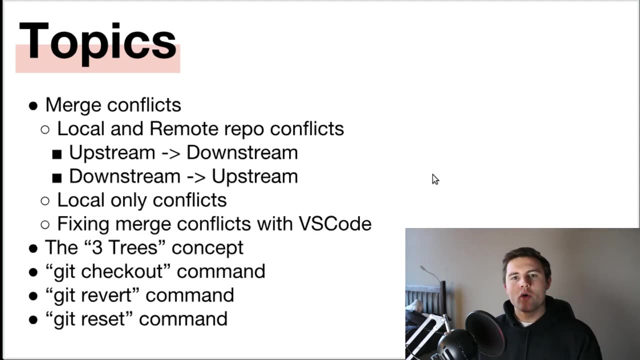 a little bit familiar with Git as a source control tool. you just need to watch video number two, because we're going to be continuing with that repository in this video And we're not going to be and working off of it. we'll be covering a variety of topics, but pretty much the main ones would be: 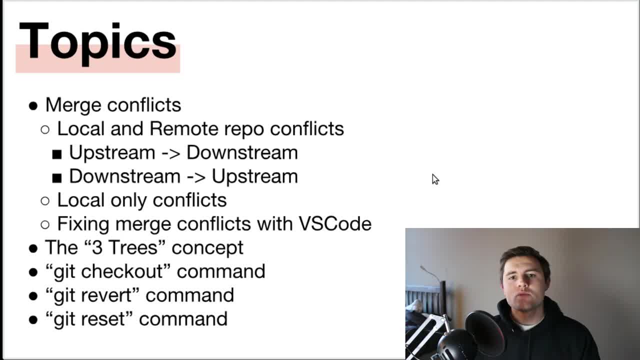 the git checkout, revert and reset commands, as well as an overview of the three trees concept that you might hear every so often. we'll start off by addressing one of the most common problems that you might face when working with git, and that is a conflict between your remote repository. 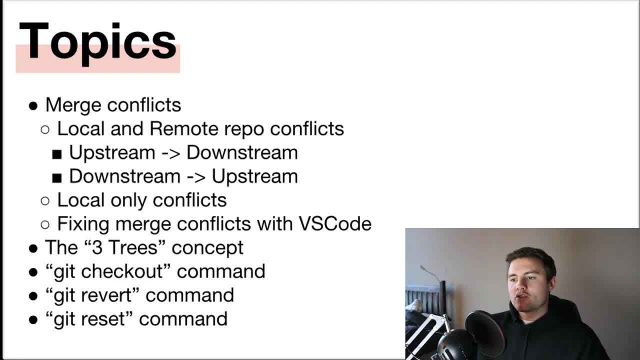 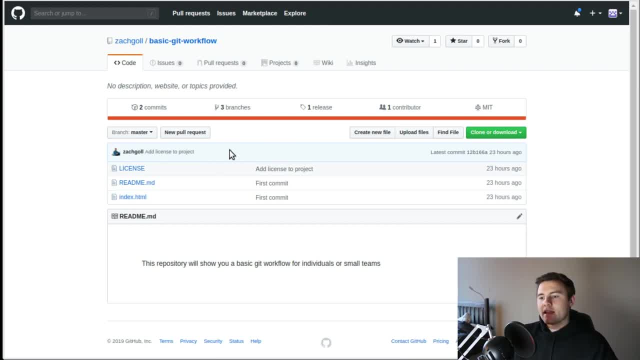 and your local repository. in order to demonstrate this, i'm going to jump into the repository that we've been working in in the last video and i've actually signed in with a different user. so you can see, at the top right corner i've got some test user that i just created and i've actually given. 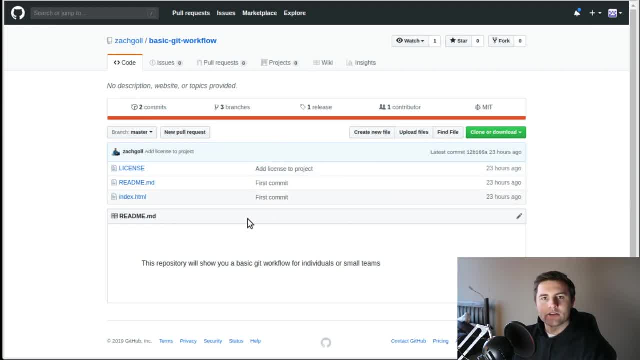 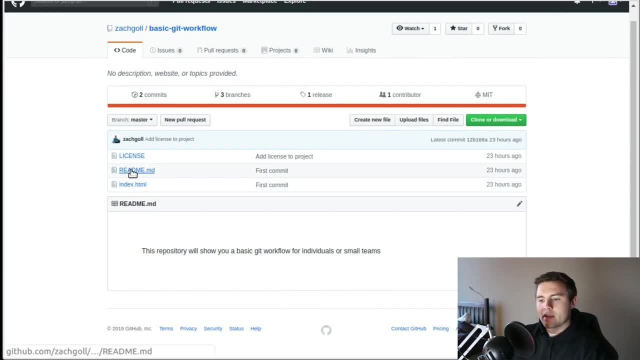 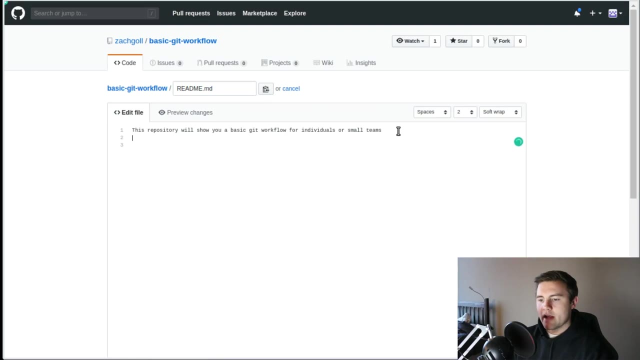 this test user access to modify the repository that we've been working in. so i'll create an intentional merge conflict. um in the readme document. so let me click into readme, edit this file and then we're going to put in a line of text here at the end that should create some sort of merge conflict. so i'll paste. 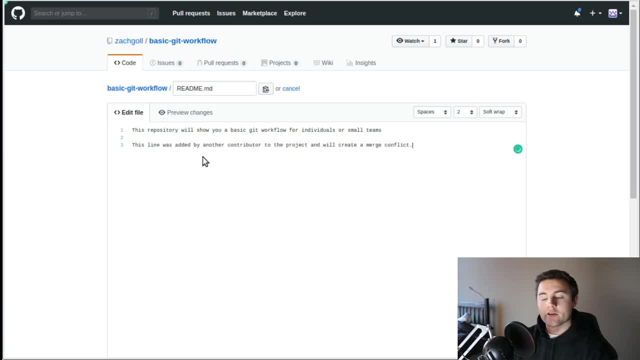 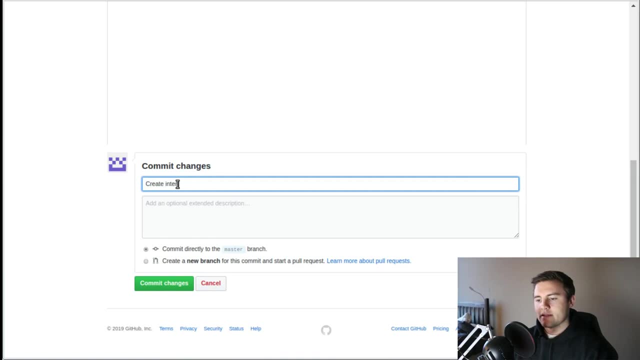 that in here this line was added by another contributor. it'll create a merge conflict and then for our commit message we'll say create intentional merge conflict and we don't need an optional description. we'll just commit the changes and, as you see, we now have two contributors to our repository. 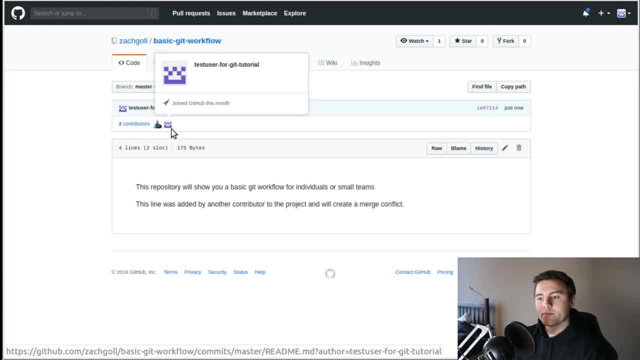 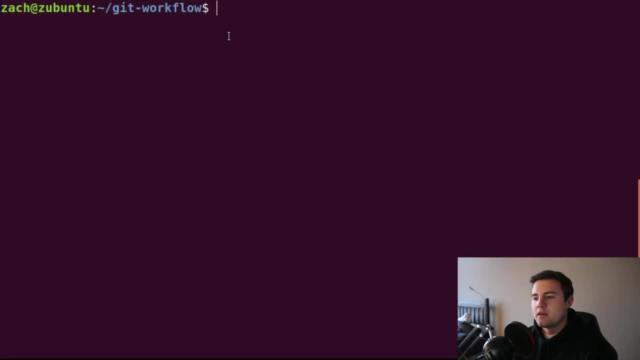 and the test user for our tutorial has been one of those contributors. now let's jump into the terminal and make a change locally. so if we type git status, we have we're on branch master, nothing to commit, working tree clean, and so therefore we can come into the readme document. 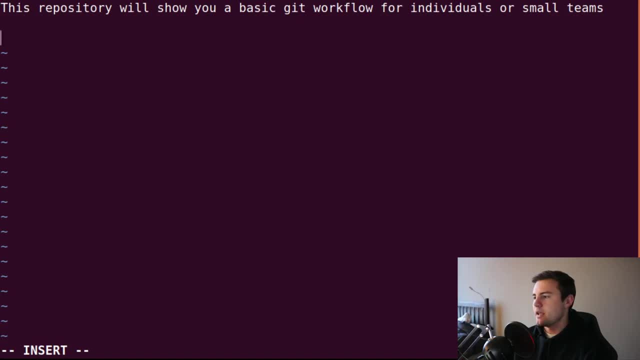 and we can see that we have a conflict with the one that we just edited with the test user and put in a local edit. that's going to conflict with the one that we just did with the test user. let me get rid of this character at the beginning. we'll save and we will quit, so at this point we. 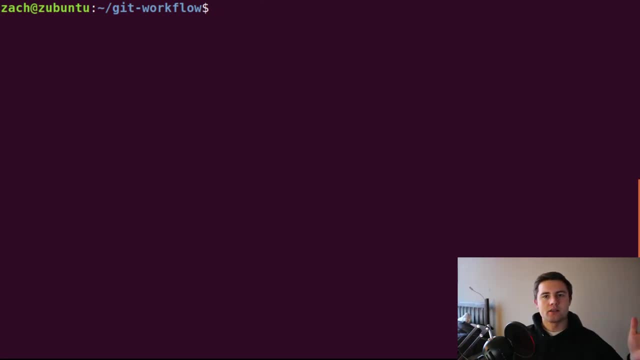 have a conflict. the readme up on the remote repository is going to be different. it has different contents than the one in our local repository. so if we were to say that we want to put in a change and we're going to do that in the master branch, we want to put in a change. 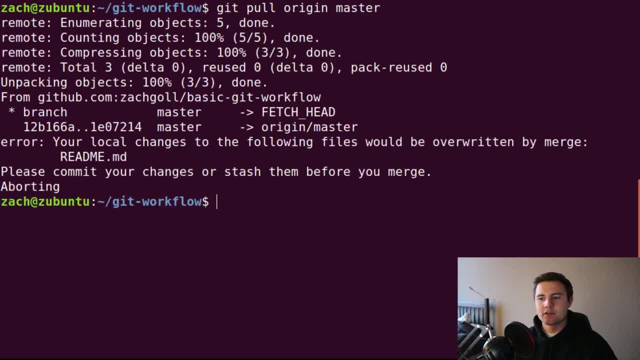 and we are going to do that in the master branch, as we've heard before, and so if we were to try to pull in the changes from the master branch, we're going to find that we have a little bit of a conflict. it says: please commit your changes or stash them before you merge, and then it says it: 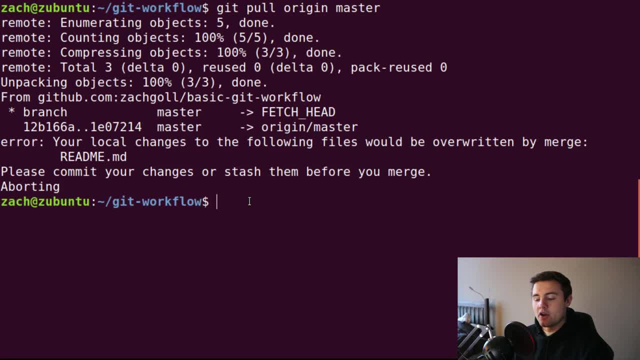 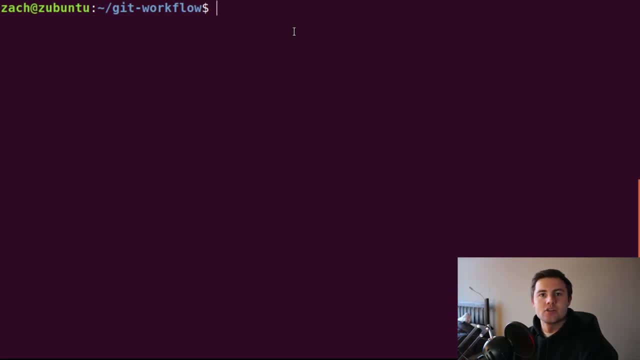 is aborting, which basically means you've got to manually fix this conflict before git can actually bring in those changes. is that we could commit our changes, as the message had mentioned? so we could, you know, add the readme and then commit those changes and then pull in the changes from the remote repository. but 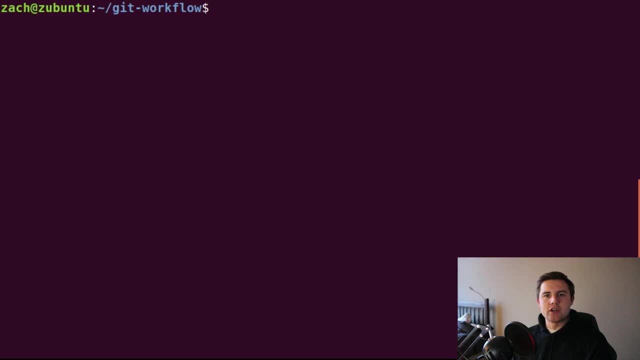 the problem with that is we'll just be overwriting our local changes. if we do that now, our second option is we could actually reset everything, so we could type this command: get reset hard flag and then head. we'll learn about this command in due time, but basically all this will. 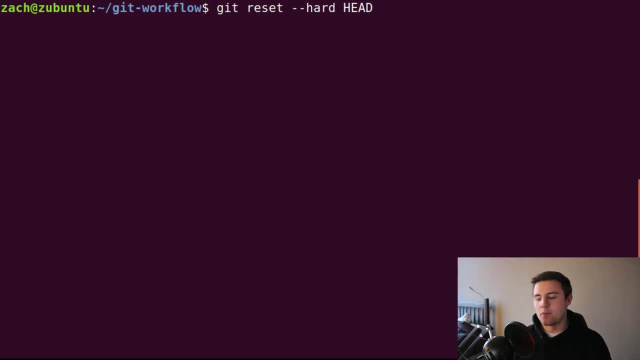 do is bring back our changes locally to the previous commit. we're not going to do that because we need to learn what the get stash command is and what this does is. it will take all of those changes that are in our working directory and just kind of stash them away for. 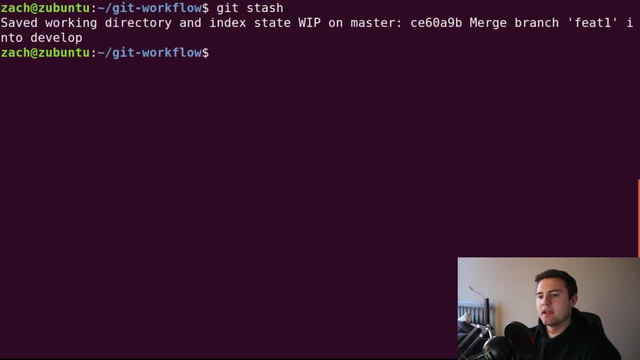 a minute. so we'll type get stash and it says it saved the working directory and it's an index state WIP on master. so there's a bunch of information here. we don't really care too much about it. what we care about is that we can now 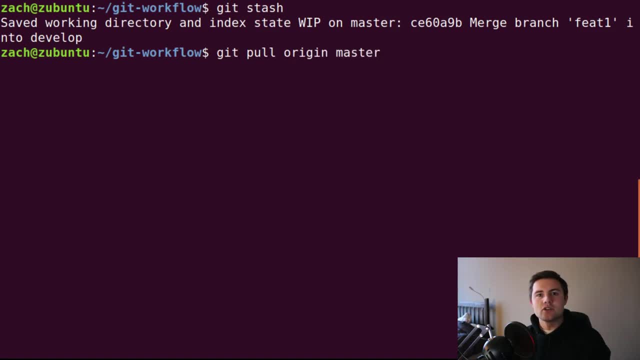 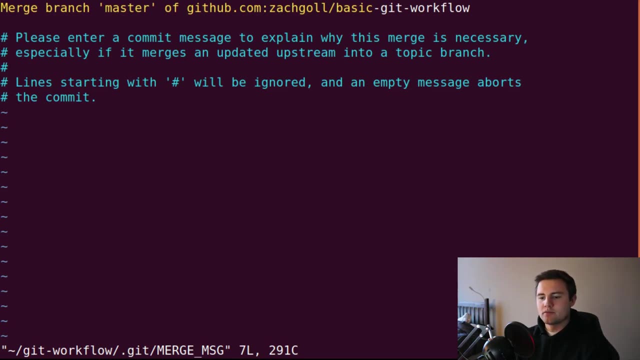 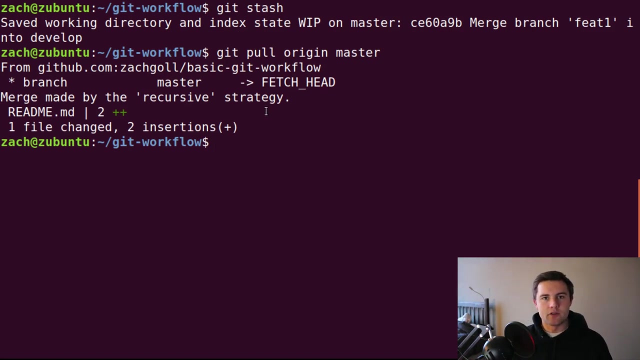 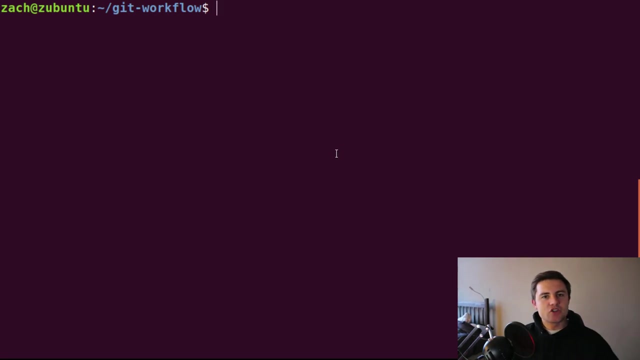 pull in the changes from the remote repository. so it'll say merge branch master and we'll just say okay, save and quit, and you can see that we have actually merged in the changes successfully. all right, so we've got these merged in. now what if we wanted to get those stash changes back? you know we had. let's see what the 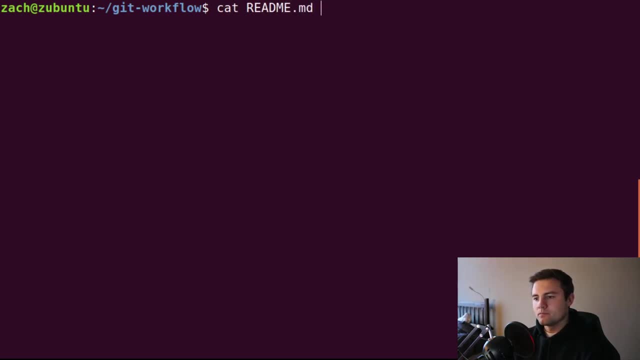 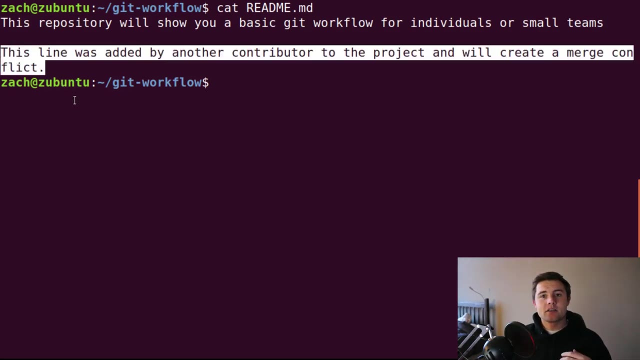 readme looks like right now and you can see that it currently reflects what we did on the remote repository and it has no recollection of the changes we made locally. if we wanted to get those changes back, we can actually get the stash back and commit that in. so first we'll type get stash list. 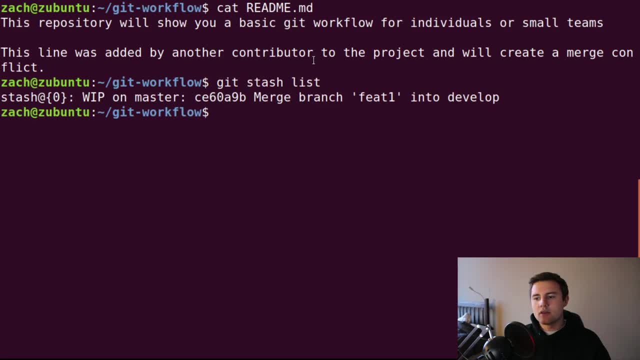 and that's going to show us all of our stash changes that we've made. you'll see that we just have one here and it's represented by this little symbol and if we type get stash apply and then give it that name, so stash- at then the little brackets zero, when we get the stash back, our workstation will still look. 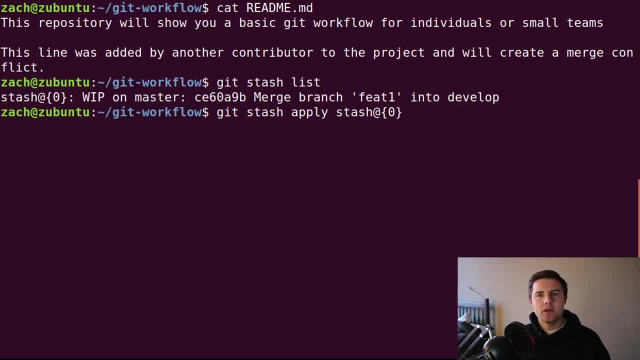 zero. when we press enter, what it's going to do is look at those stash changes, take those changes and overwrite our current repository with those changes. let me press enter. you'll see that we have a merge conflict, but this should be okay. let's cut out the readme and we now see that. 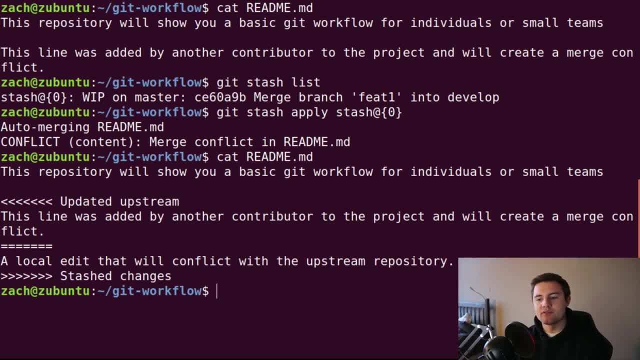 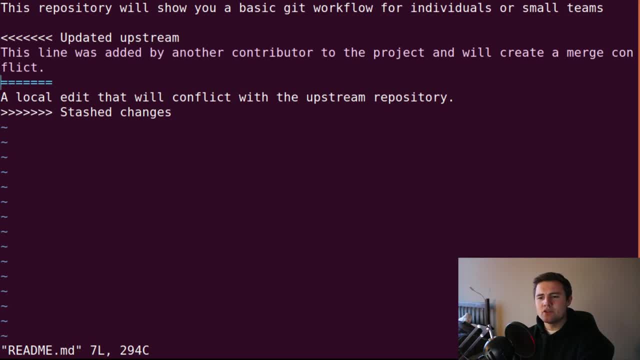 there is a few extra lines of text within this file. we need to go into the readme document and resolve this merge conflict and all we need to do to resolve it is delete this line, delete that line, this one and this one. so now we have our stash changes and we can save and exit. 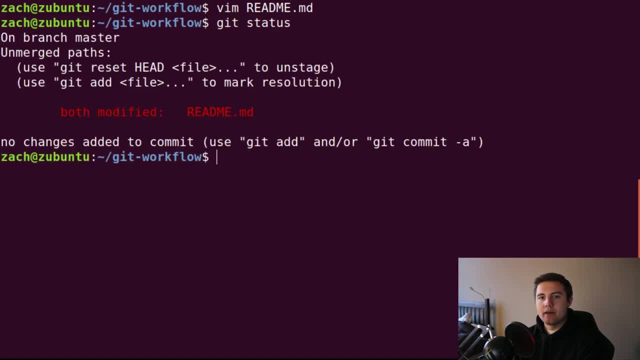 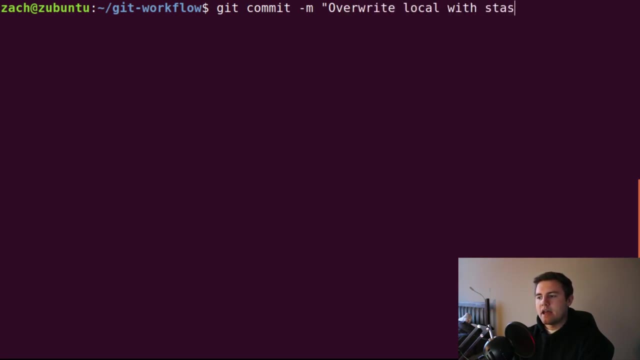 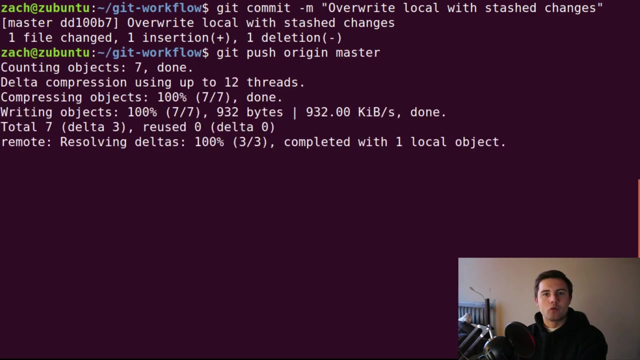 and then we'll type: get status, we have something modified so we can add that, and then finally we can commit and and overwrite local with stashed changes and then we can finally push that to the remote repository and we have successfully taken those stashed changes and overwritten, uh, what we had pulled in from the remote repository. now you might. 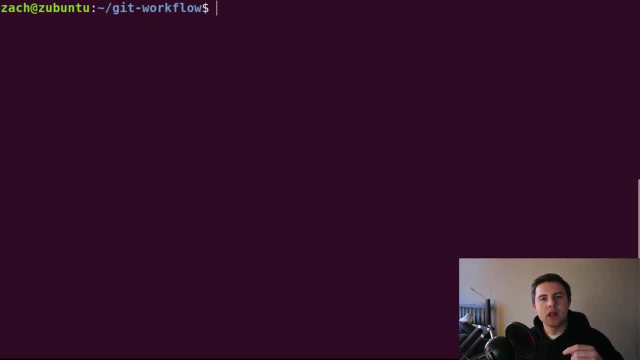 have noticed that the second time around when we went to apply our stash changes in the local repository we actually had a theme change- you might've seen in there showing up in our storage repository had a little bit different process. So when we pulled our changes from the remote it didn't ask us to resolve any. 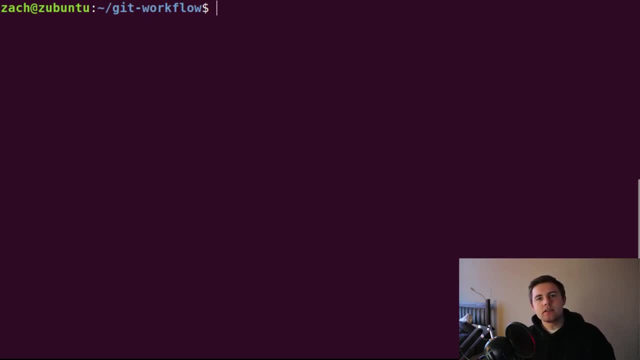 merge conflicts, And that is because this is a slightly different conflict that we're dealing with. So before we looked at a conflict between the remote repository and the local, and in this second case we were looking at a conflict between just the local repository. I'm going to demonstrate this again. 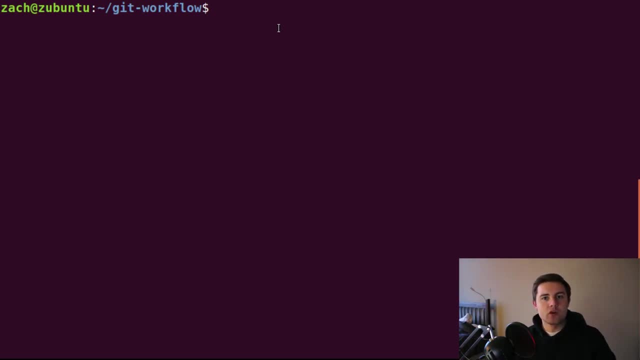 but this time around we're going to use the Visual Studio Code editor to resolve this merge conflict, And I just wanted to introduce this because I know a lot of people work in Visual Studio Code. It's free, it's an awesome text editor and I work in it myself, so I wanted to leverage. 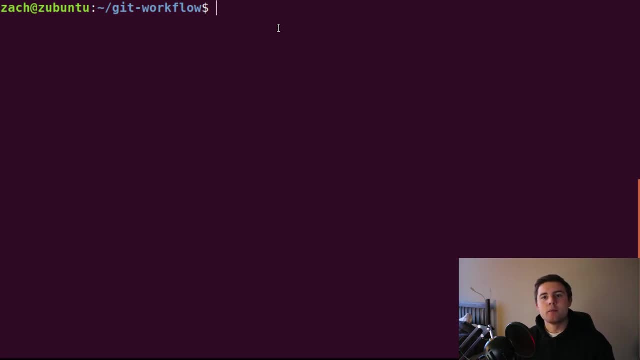 the capabilities of it and kind of show you how easy it is to resolve conflicts in it. First we need to create a conflict. So what we're going to do, let's type in git status: We've got a clean repository, so that's good. 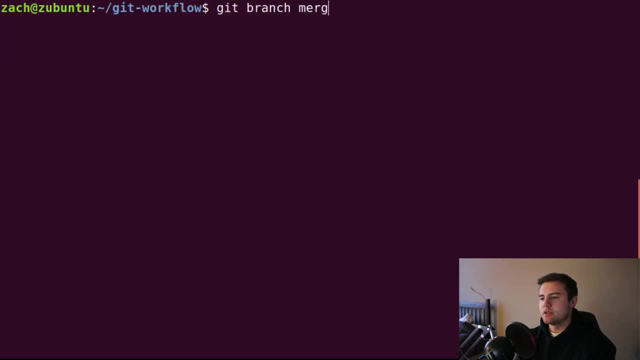 I always want to check that first, And now what we're going to do is create a merge conflict branch. So if you remember from the last video, this is the command we used to create a new branch, And then the checkout command, which we'll explore a little bit. 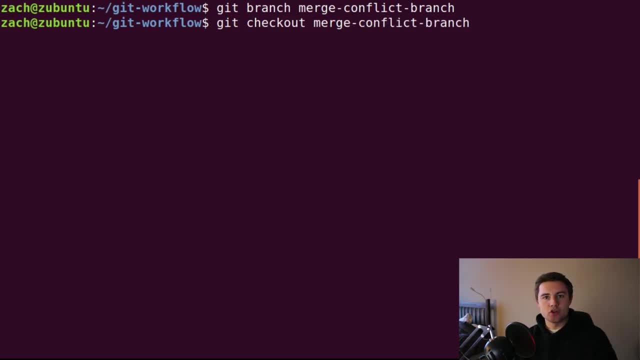 more later is going to be how we actually switch over to that branch. So at the moment, we can see that our readme file has the following text: So we need to edit this using vim And instead of that line we're going to say: I made this. 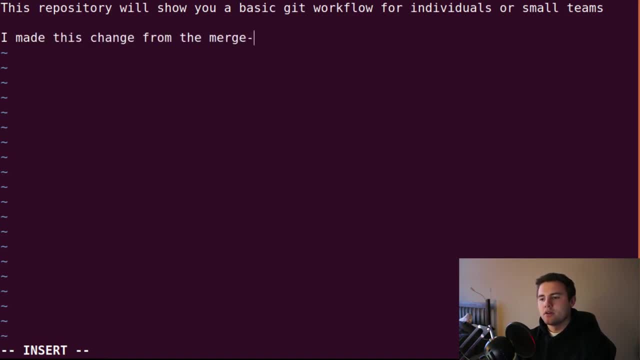 change from the merge conflict branch. if I can type Currently, if we were to try to merge the conflict branch into the master branch, it's actually going to be okay And although the contents of the readme is different, we haven't actually made 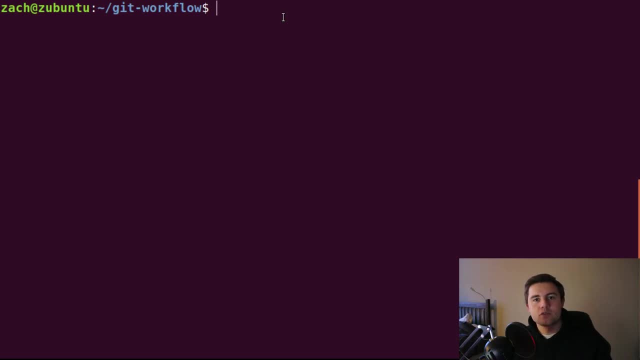 any change in the master branch. So what it's going to assume is that we just want to overwrite the changes from the master branch with the incoming merge conflict branch. If we really want a conflict, we need to make a change to the readme in the master branch, So as 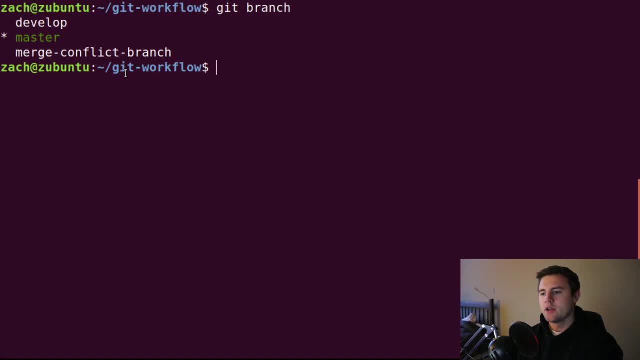 you can see- we've already checked that out- We're on the master branch, So all we need to do is go in vim and make some sort of edit. Let's just say some conflicting text from master branch And we'll save and quit. We will add. 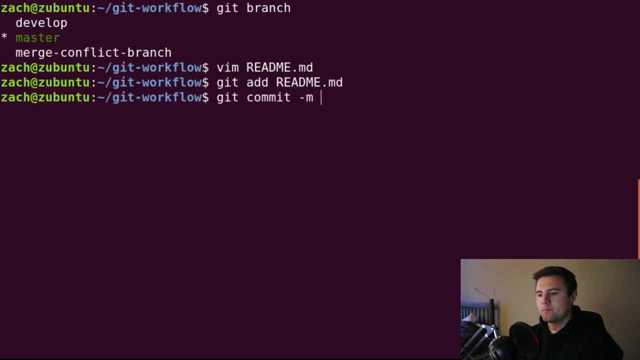 those changes, commit them, and we are finally ready to actually merge them in together and fix the conflict. So we'll type git, merge, merge, conflict branch. And so remember we are on the master branch right now And so therefore, whenever we type, 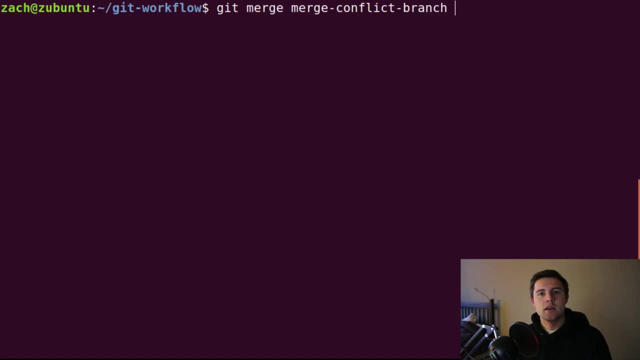 git merge, it's going to bring in whatever branch we're specifying into the current branch that we're on. So I'll press enter and it'll say auto merging conflict. automatic merge failed. So this means that we have to manually resolve those and commit them on our own, And in this case 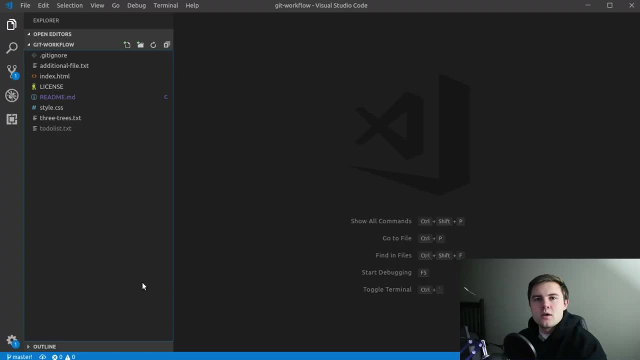 we're going to use Visual Studio Code to do so. We are now in Visual Studio Code And to get to this merge conflict, we can either click on the file that we know is the actual conflict- We know that it's the readme- Or we can 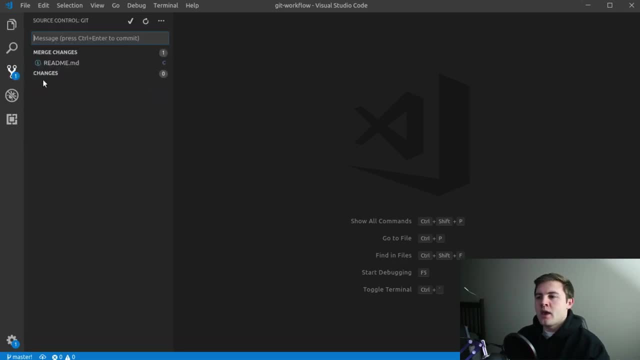 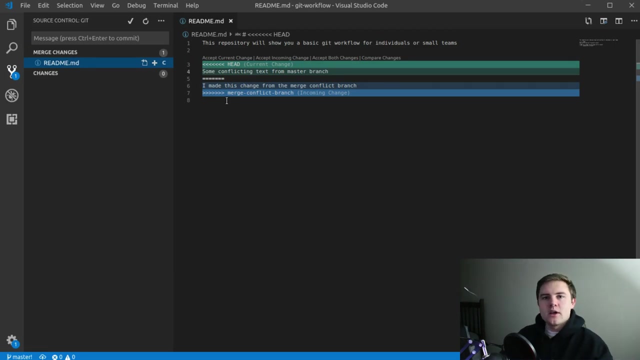 come over here to the source control tool And it'll show some merge changes that we need to address. So we can double click the readme to open it up And you'll see that we get this nice little highlighted area which basically lays out what the incoming commit is going. 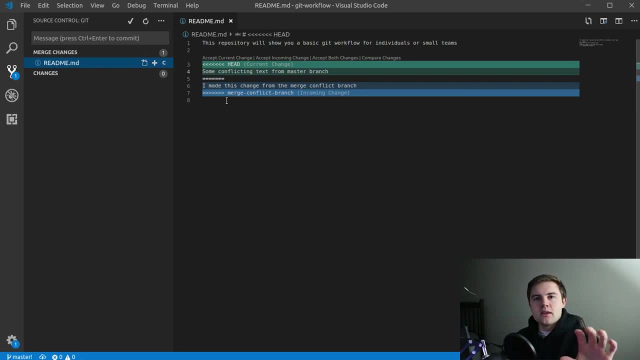 to be So, the text that we made in the merge conflict branch And what the current change is, In other words, what we made changes to in the master branch. So we can accept the current change, the incoming change, both, or compare changes In this case. 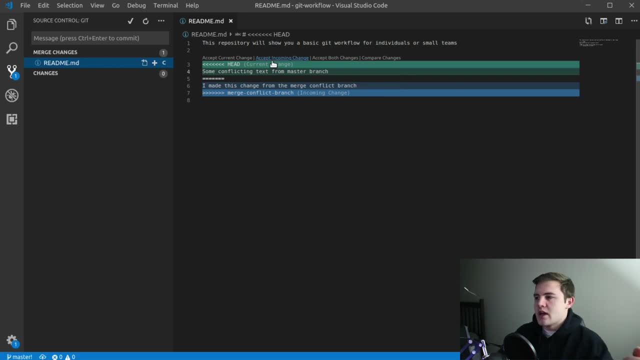 we just want to accept. maybe the incoming change Doesn't really matter, And when we do this it's going to delete the current change and pretty much resolve the merge conflict for you. So right there, we resolve the conflict. We'll control S to save the file. 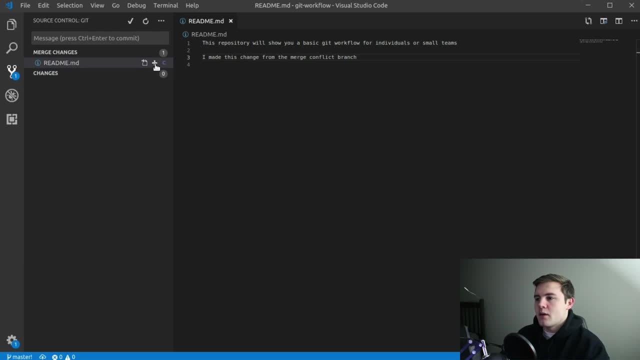 And then we have two steps left. Pretty easy. Come over here and press this plus button to stage the changes. This is the equivalent of running the git add command. So press that, We've staged it. And then finally click this check mark up here to commit the change. 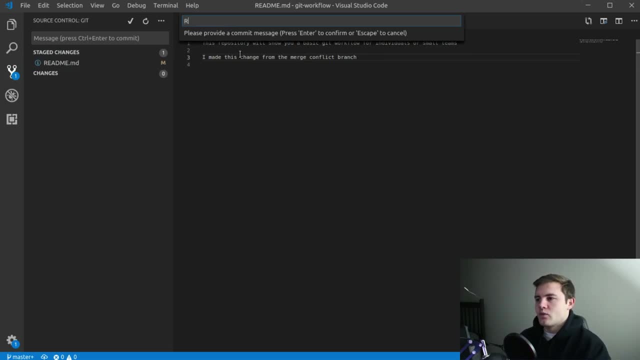 And we can say: resolve merge conflict. And that will be our commit message when we press enter. So we pressed enter And everything has been committed And we now have resolved that merge conflict. So this is just how you would use Visual Studio Code. And the real power of this comes in when 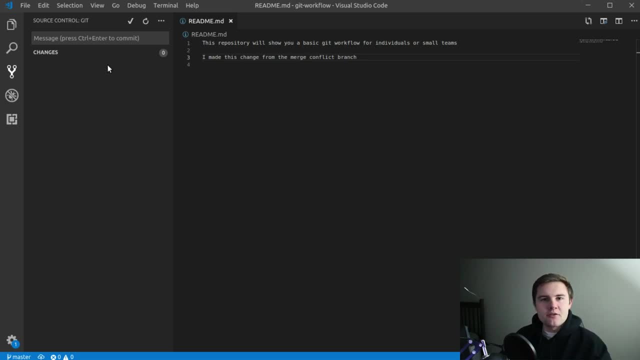 you have multiple merge conflicts. Maybe you have ten different files that you have to resolve. It's really easy to just click this little source control tool and then look at all the files that you need to address and just start clicking through them and accept the changes that you want. 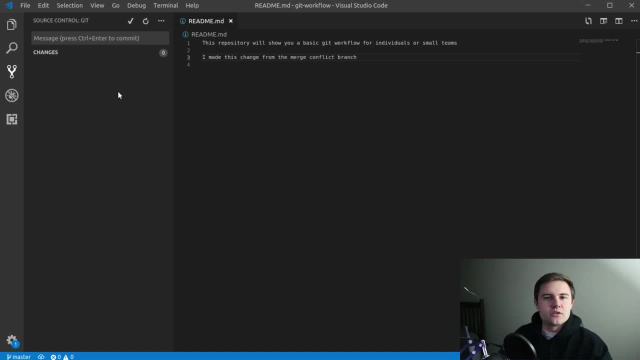 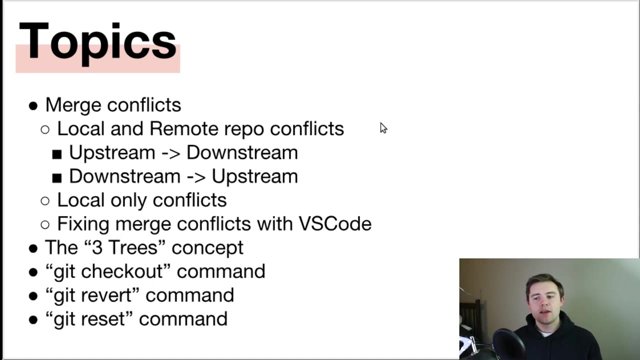 So that's just a really neat tool that I thought would be useful to show and hopefully you got a little bit out of it. To this point we have covered how to fix a merge conflict And that is a huge sigh of relief to a lot of people, including my previous self. 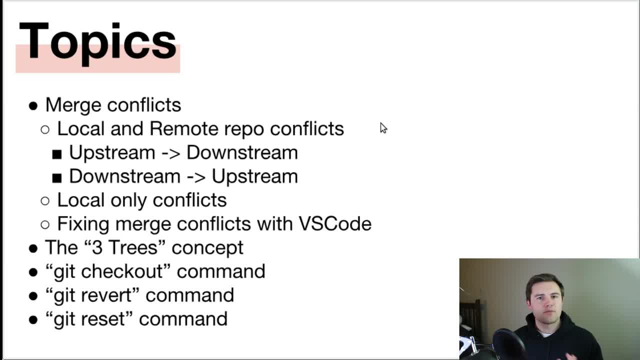 I had a pretty hard time with this whole concept. I thought it was so much harder than it actually was And every time I had a merge conflict I thought it was the end of the world. I had to restart the whole repository and it was just a mess. So hopefully that helps. 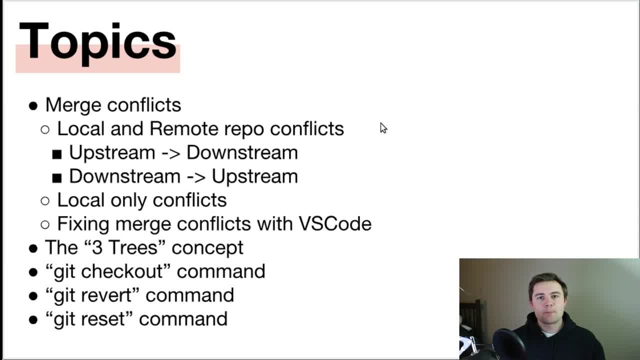 you kind of feel a little bit more comfortable using git. The next couple commands that we're talking about- the git checkout, git revert and git reset commands- they all have something to do with kind of moving around in your repository and editing the current state of it. Now. 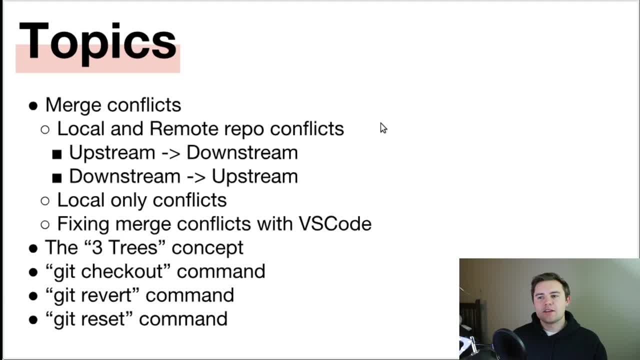 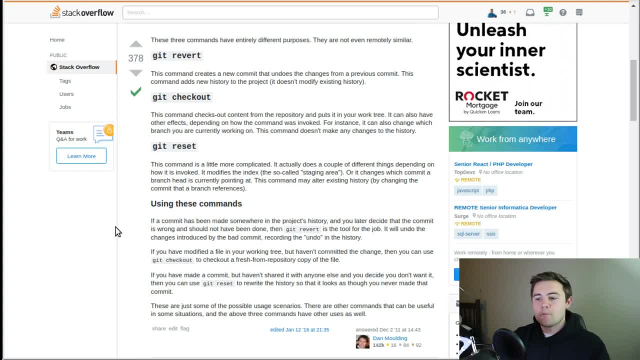 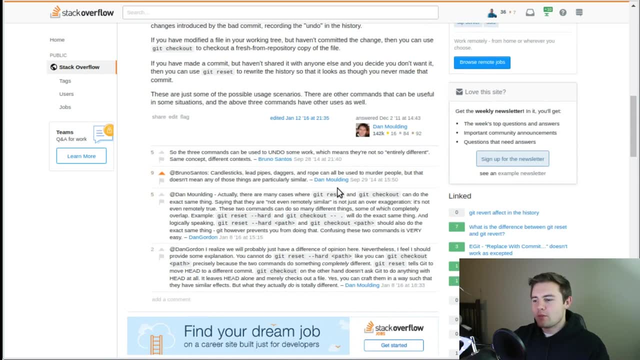 these commands are very similar and you can actually. we'll come to this stack overflow post that I stumbled upon. that, I think, explains it pretty well, And there's actually a comment down here. I put a like on it. It says lead pipes, daggers and rope can all be used to murder people. but that doesn't mean. 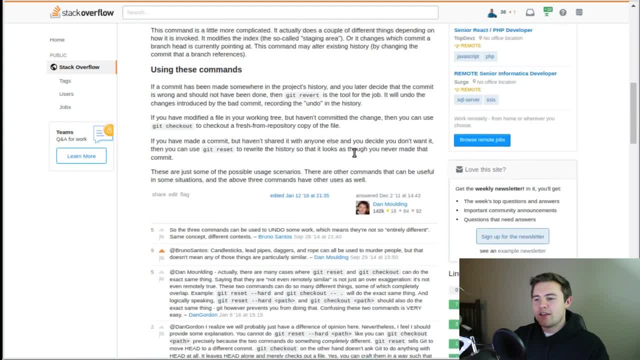 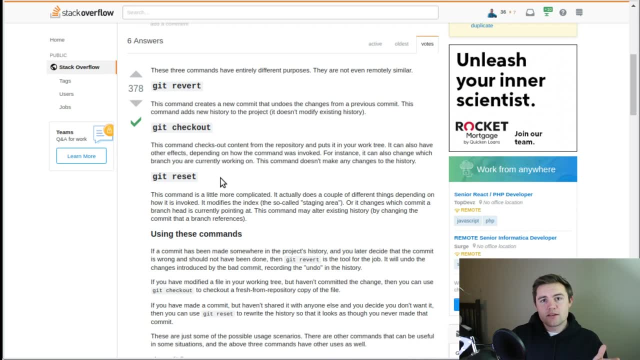 any of those things are particularly useful, And that's a pretty good analogy for these three commands, because they definitely can do similar things. but there are some specific situations that one is going to be better than another And I'm going to show you which situations warrant which command. But first, 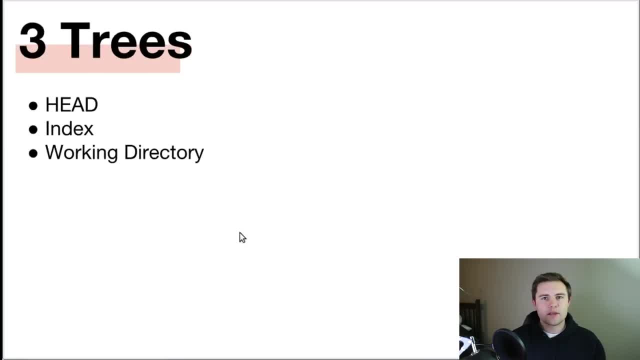 we need to understand something called the three trees, And if you type this into Google, this is what you're going to find. The three trees of git are head, index and working directory. Now, what does that mean? Well, before we try to explain all of that, I think that we'd 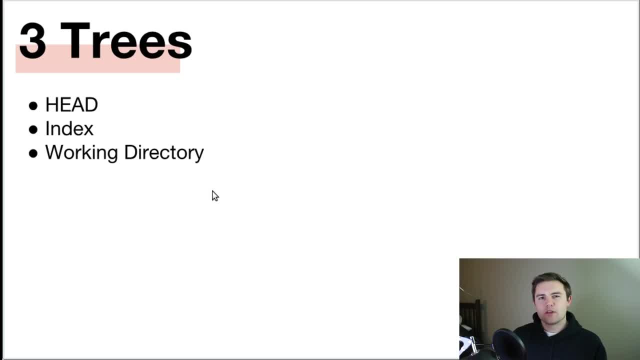 be better off to look at these three trees with a little bit different terminology, And that is the repo, staging area and working directory. This is a little bit more simple to conceptualize and it's more in line with what we've been learning throughout the last video. 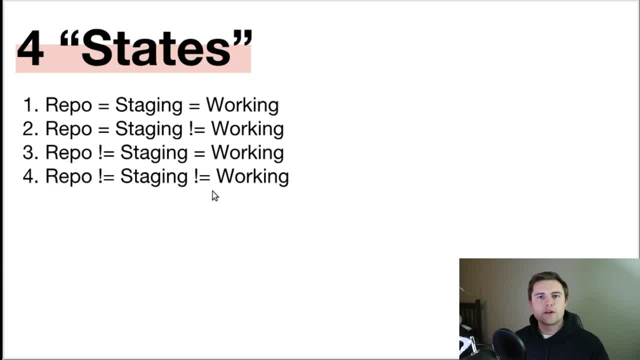 So basically, these three trees can have four different states at any given time. You can have all of them equal to each other, all of them not equal to each other, and then some sort of combination here. I know this doesn't make any sense right now, so we're going to jump into the terminal. 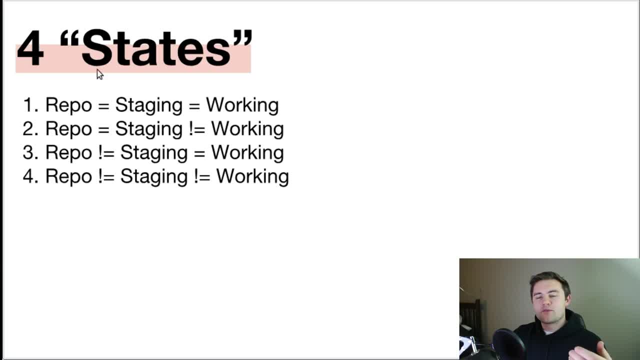 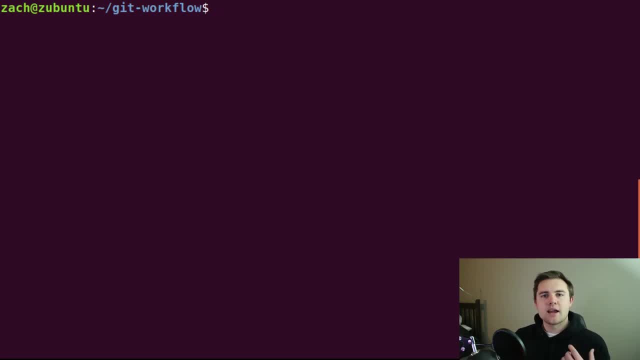 to recreate what these four states represent. The first state that we'll find ourselves in is state number one, And this is kind of the one that you're always going to be seeking, and you definitely want to make sure that you're in state number one before you go running a bunch of 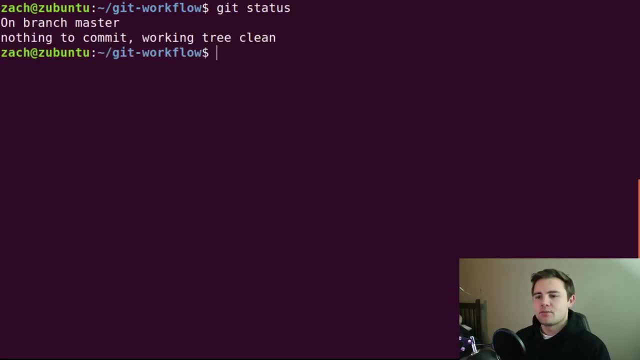 commands. So if we write git status, you'll see this message that we're pretty familiar with. at this point It says nothing to commit. working tree is clean. This is always going to indicate to you that you are in state number one, or in other words, 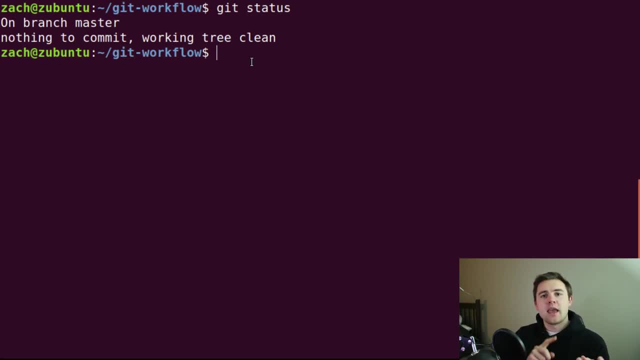 the working directory, the staging area and the repository are all going to be synced up. So that is state number one. Now what if we wanted to create a different state? We can do this by creating a new file, So we'll type 3treestxt. 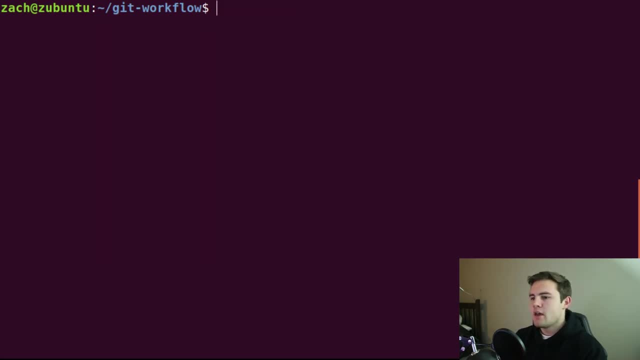 and we don't really need to put anything in that file right now. All we need to do is type git status again, and this time you'll see that we have an untracked file. So at the moment we have a divergence between the working directory. 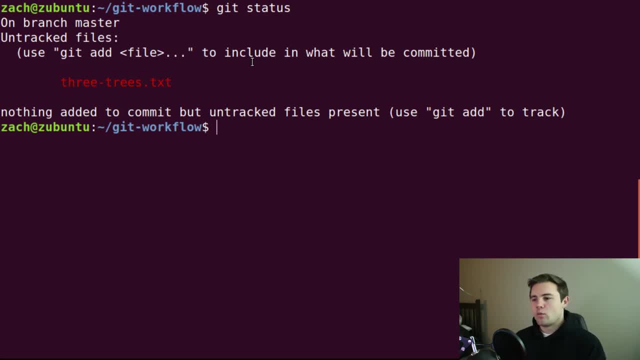 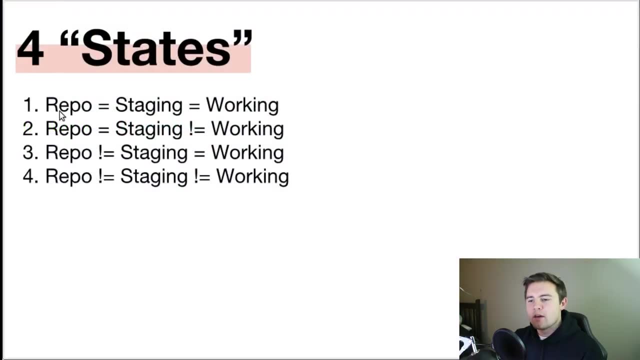 and the staging area. So we'll go back to our slideshow here for a moment and look at the current state that we're in. So we're definitely not in state number one, because we had already looked at that. Now let's go to. 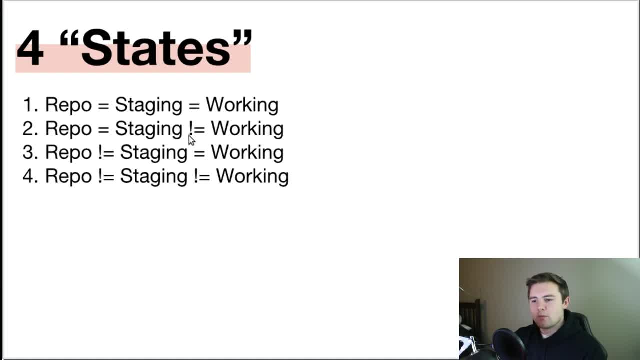 state number two. It says repo is equal to staging. but staging and repo are not equal to working And that fits the bill pretty well because the working directory has this new file that we haven't quite added to the knowledge of the git tool and the repo. 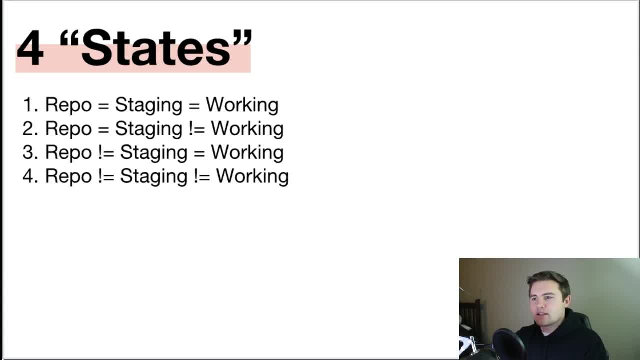 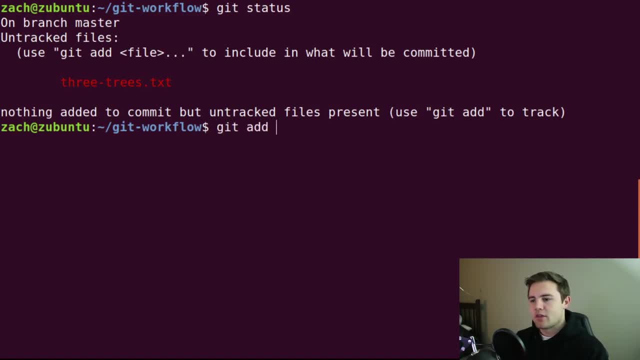 and staging are going to be similar. So we are now in state number two. Alright, so we'll come back to the terminal and type git: add threetreestxt. Once we do this, we'll type git status again, and now you can see that the git 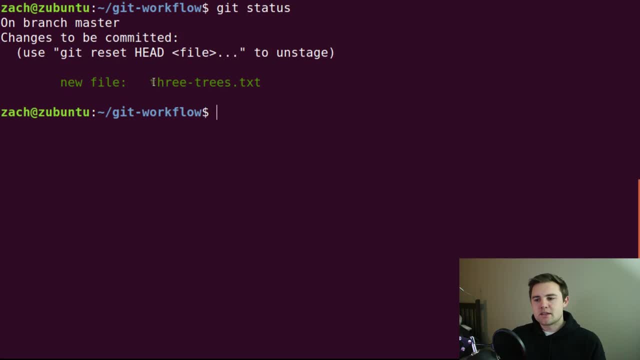 utility has picked up on this new file and it realizes that we have added it to the repository. Now we haven't yet committed to it, committed to the repository. so basically, right now our working directory is synced up with our staging area And this little area right here. 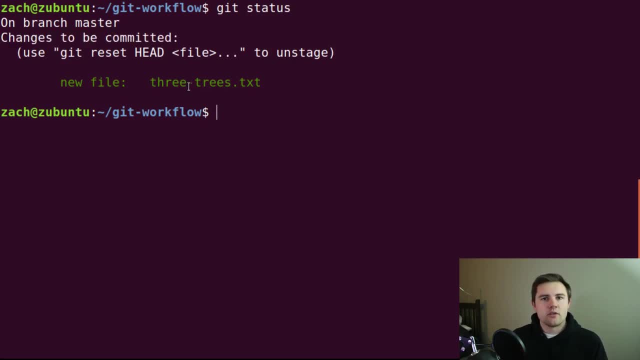 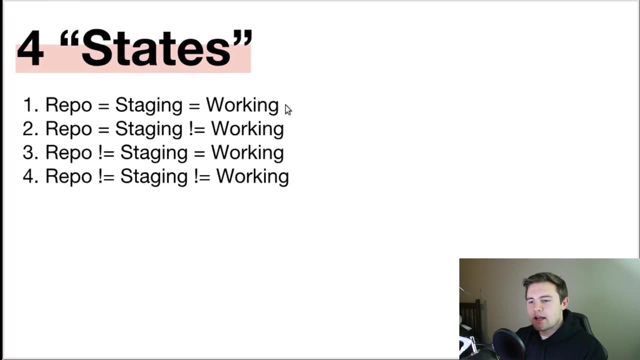 under the changes to be committed. that is essentially what we call the staging area. So go back to our powerpoint once again and you see, we're not in state number one nor number two, we are in state number three. So staging and working are equal and the repo is the only. 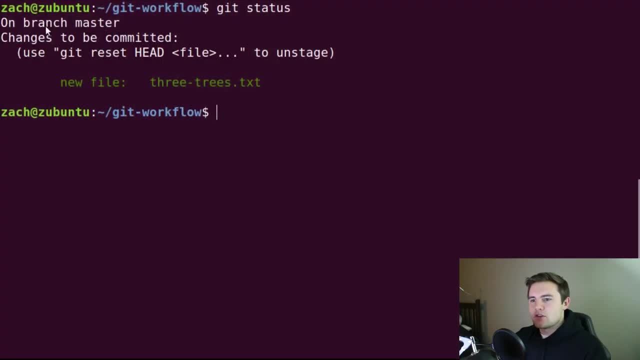 thing that is different. So, finally, we will come back to the terminal and what we can do is commit and add some message and once we commit that, then we're going to be thrown back to state number one, where everything is synced up. I'm not ready to commit this change. 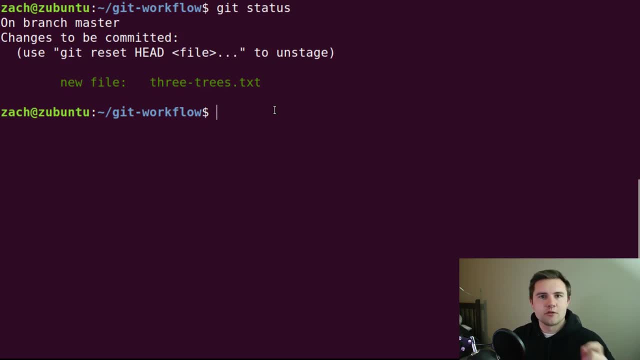 just quite yet, because I want to throw us into state number four and demonstrate how we could have all three of these trees unequal to each other. And the way that we do that is by just creating an additional file. So we'll say additional file, dot text and then we'll put some random 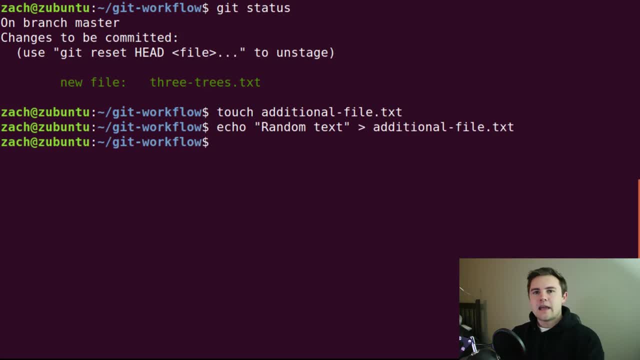 text in there And at this point we have state number four. Now, how do we tell that we are in state number four? Well, we can clear the screen and type git status. and now you can see that the staging area where we see changes to be committed. 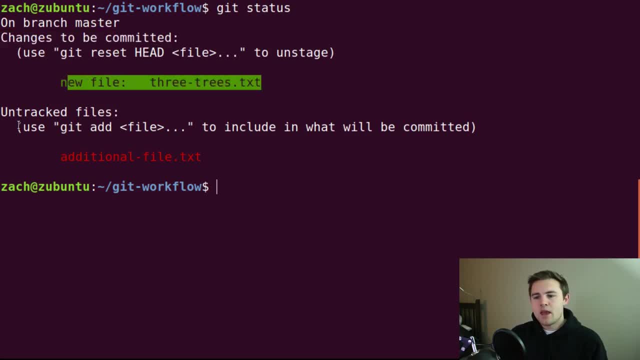 that is, the staging area, has one file in it, and then the untracked files, which represents the working directory, has this additional file And neither of these files are in the repository. So in other words, we have state number four, where nothing is equal to each other. 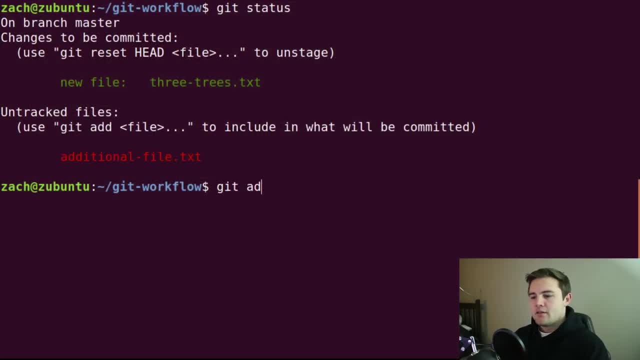 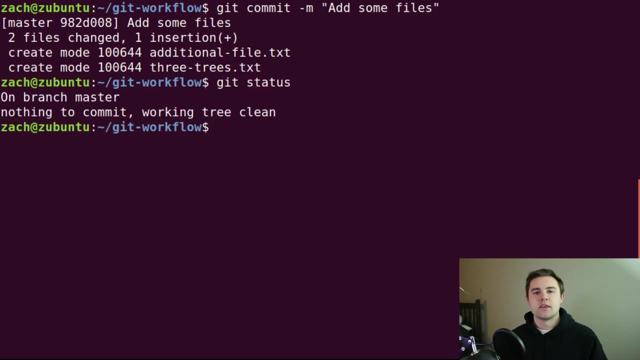 Finally, we can add the additional file, clear the screen, commit that and then, finally, we are back to state number one, where our git status returns that the working tree is clean. As we move along through the rest of the commands, I want you to always 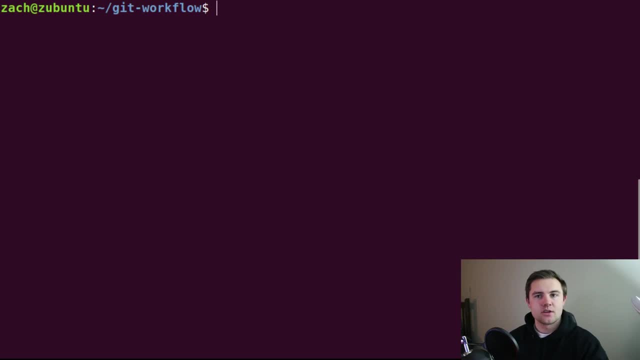 keep at the top of your mind what state you are in. So I know it's going to be a little bit tough. since you just learned it, I'll try to point it out as we go along. but what state you are in will affect the commands we're about to run pretty dramatically, So it's important. 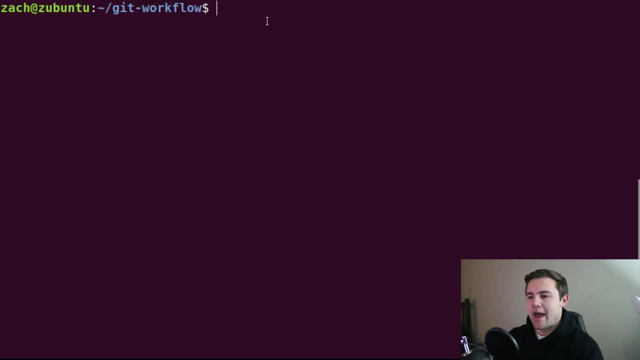 that you always keep in mind what current state we're at. Now. the first command we're going to be looking at is the checkout command, So we've already covered this a little bit. I just wanted to show you a few subtleties and show you more conceptually what's going on. 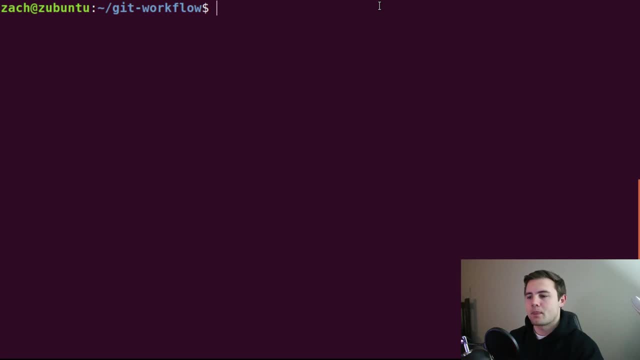 when you checkout a different branch or commit. The first thing that we'll do is start to get used to using the git log utility, because you're not always going to have someone putting together a PowerPoint to visualize what a repository looks like at a given point in time. 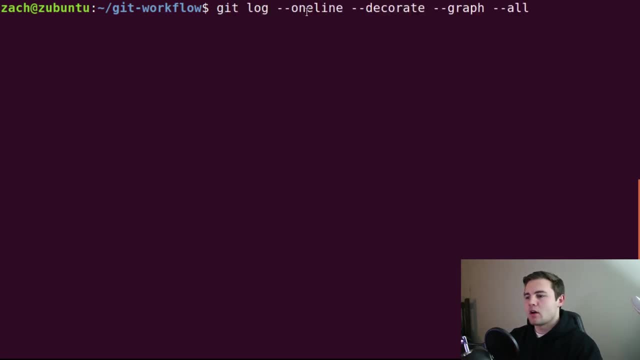 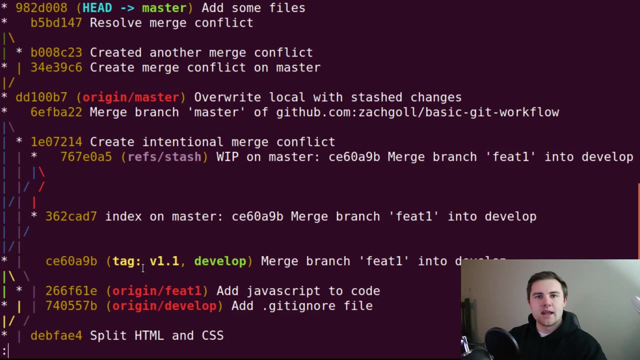 So you can type this command here, the git log and then all these little options, and this will show you what your repository looks like at any given moment. You can see that our repository is pretty complex. We've made quite a few changes at this point and you can just 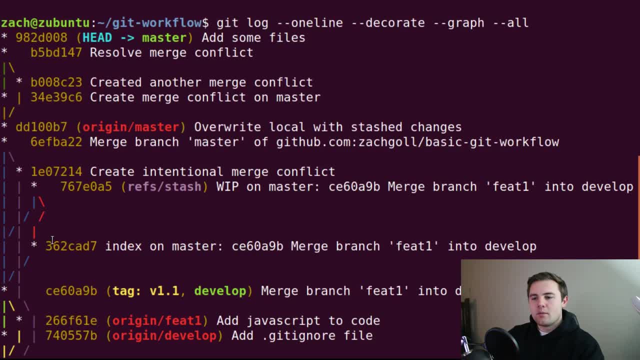 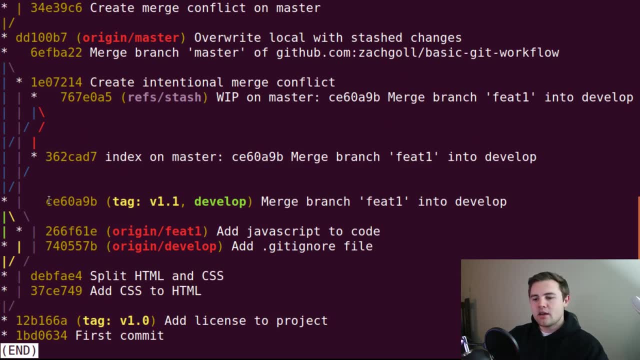 press spacebar to go down to the end. What we're going to look for in this particular scenario is where the develop branch is at, And you can see where the develop branch is back at the version 1.1 release or commit: CE60A9B. 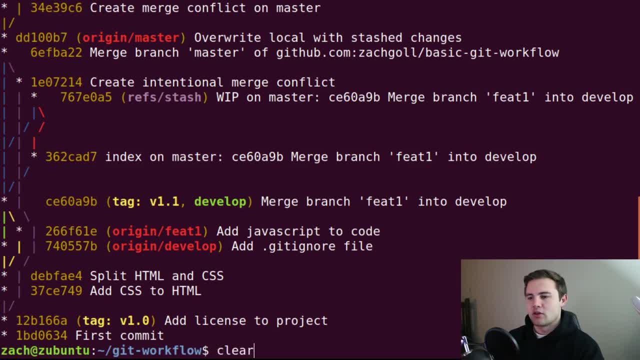 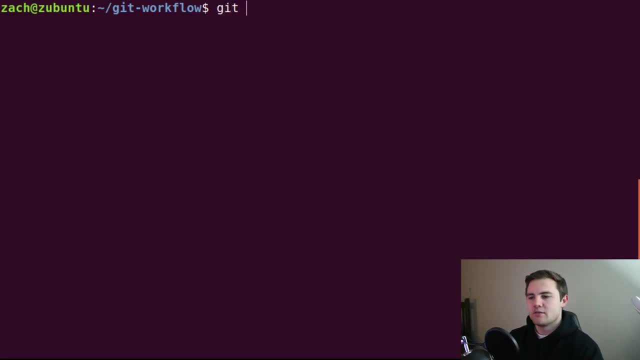 So we want to go back to that particular commit or the develop branch. The way that we'll check out the develop branch is by typing git checkout develop, And you already know this. but let's remember what state we're in, So currently we should be in state. 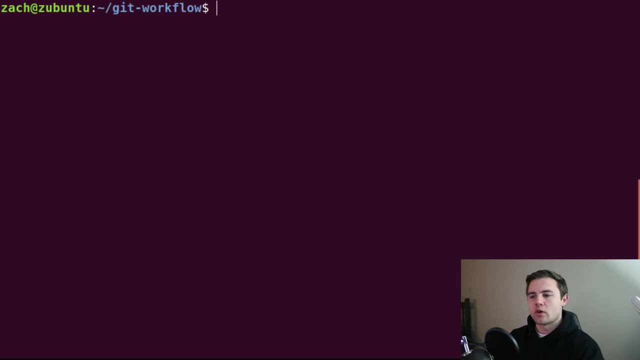 number 1, which is good. That's where we want to be when we're about to run the git checkout command. So we'll check out the develop branch, And what we just did was we switched the head pointer to point at the develop branch pointer, which 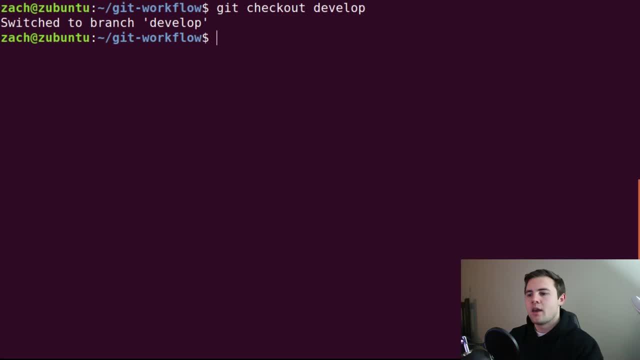 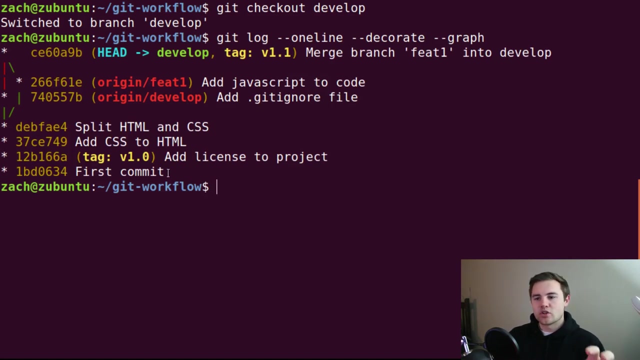 points at the version 1.1 release. And if we run this log command again and take off this last flag, that says all it'll only print the history of the develop branch. You'll see it's a lot less for us to look at which is really useful And we can. 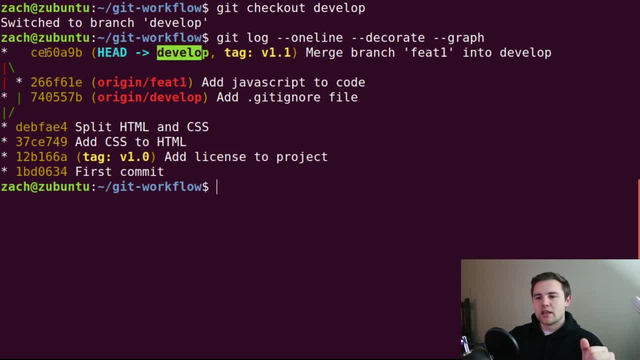 see that the head is now pointing at develop, which is the latest commit on that branch. You'll also notice that we are still in state number 1.. So if we type git status, we're on the branch develop and we're in state number 1.. Everything. 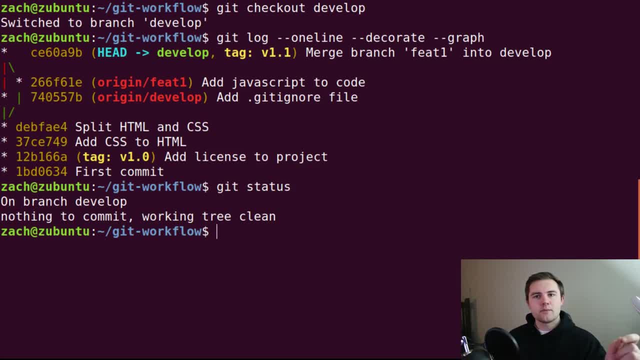 is synced up. So although we changed the head pointer, we didn't actually change anything about the repo or the working directory or the staging area. Now what if we wanted to maybe check out the first commit in this entire repository, Or at least the first commit of the develop branch? 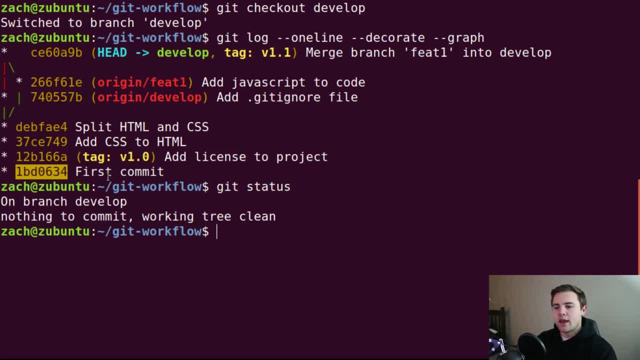 That would be the 1BD0634 commit, and I just know for a fact that this was the first commit of the entire repository, So if we wanted to check that out, it would be as easy as copy and pasting this abbreviated commit hash into the git checkout command. 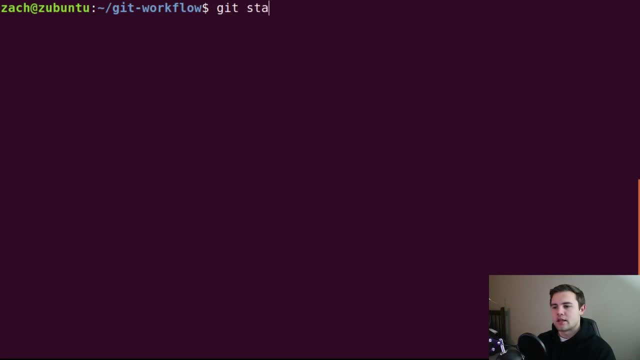 So we'll type: we'll first make sure that we are in state number 1, as we always do, and then we can type git checkout and then paste in the abbreviated commit hash. It'll say: we are now checking out this commit and you'll get this. 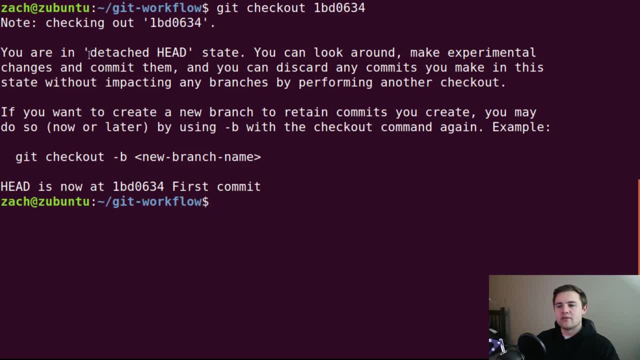 message that says that we are in the detached head state. Now what does this mean? Basically just means that the head pointer is no longer pointing at a particular branch, it's pointing at a lone commit, And this is basically telling us that if we want to work on anything, 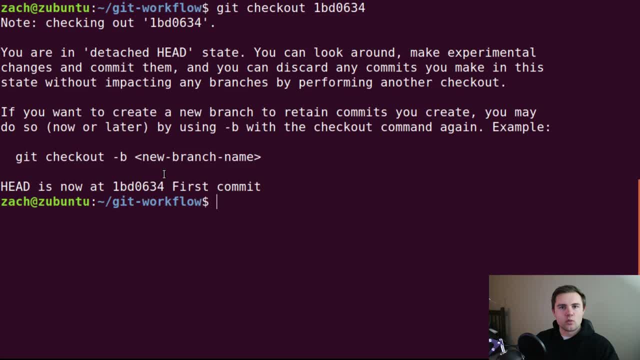 from this point in time, we need to first create a branch that we can commit the changes to. We're not all that interested in doing this, so let's just take a quick look at what our repository looks like visually. So I'll go. 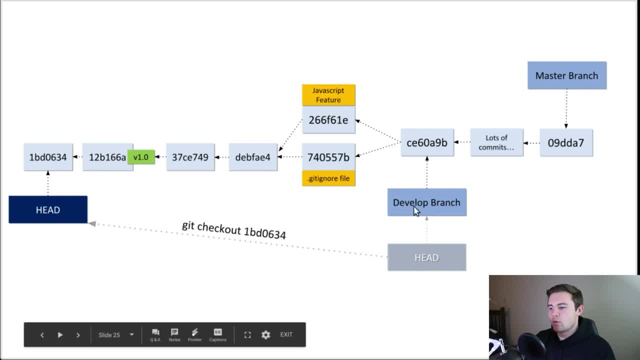 back to the PowerPoint and you can see that we were originally pointing head at the develop branch and then we checked out this first commit, And so basically what happened is the head got moved over to the first commit and we're no longer pointing at any of the branches in the repository. 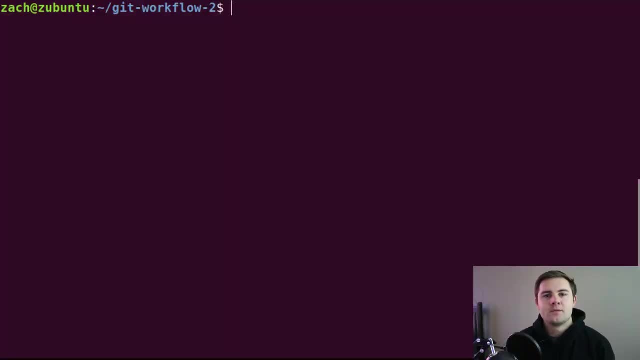 We will now talk about the git revert command. This is one of the more challenging commands in git, but once you understand the concept behind what it's doing, it's not actually that complicated. It's basically you can think of it as like a big undo button And the feature about the 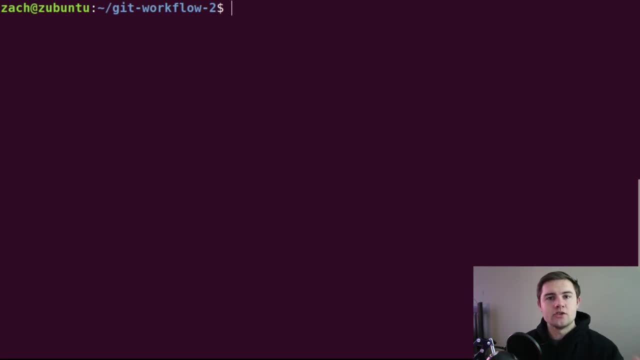 git revert command is. it's not only an undo button, but you can undo the undo that you just did. So in other words, we're actually going to commit a brand new commit in our repository to reflect the undo that you had just done. I know I'm kind of talking in circles. 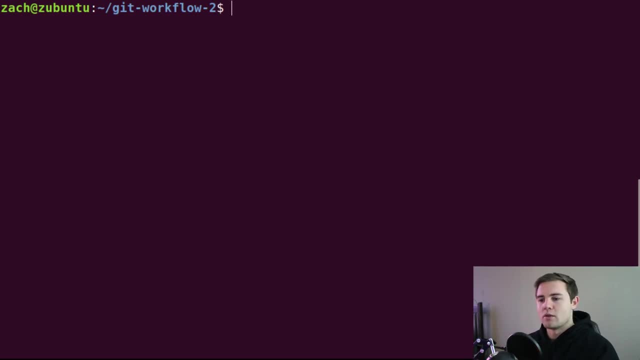 so let's jump into it and you'll kind of start to see what I'm talking about. So, for this example, I've created a brand new repository that mirrors the repository we've been working in. If you log out the contents of it, you'll see that it's just a lot more. 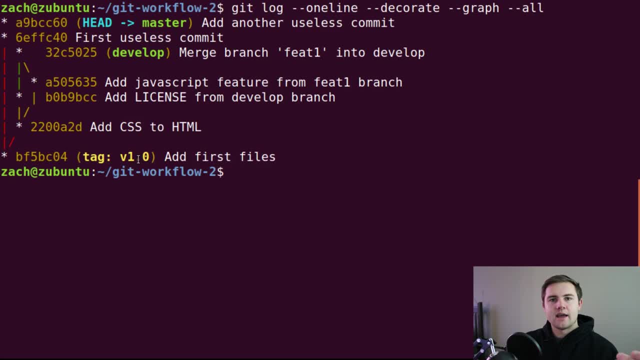 simplified. We have our first release at tag version 1.0.. We made a commit where we added CSS to the HTML. Then we branched out into feature one branch and develop branch and worked on some stuff, Eventually merged those two together into the merge commit. Then we made two commits. 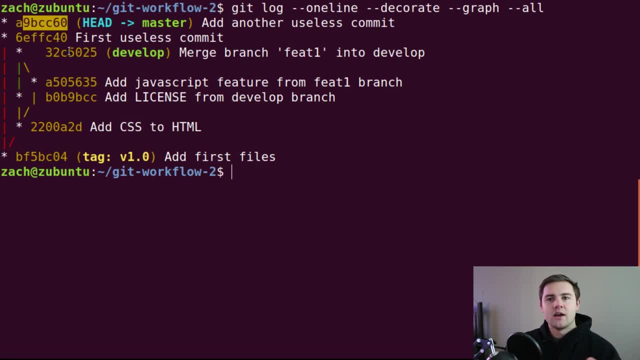 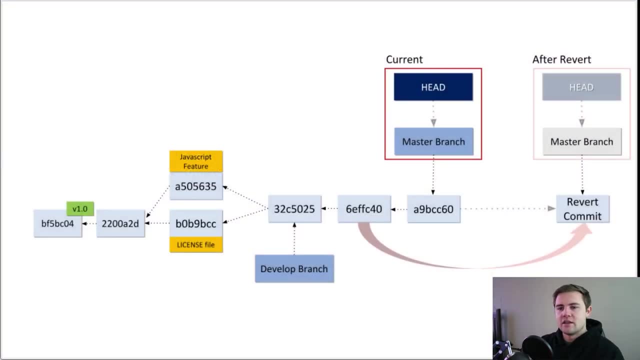 here later that were useless and will eventually kind of either revert back from or delete entirely. I think it'll be easiest if we look at this in the visual again, And this is where we start to understand what I was talking about with all this undo of the undo. 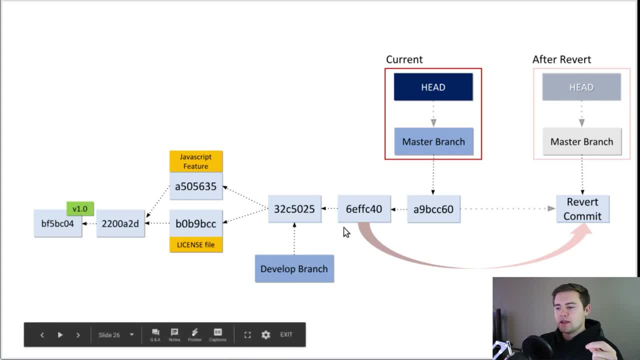 So, basically, if we wanted to revert back to the commit 6EFFC4O, which is the commit previous to the one that we're currently on, all we're going to do is take the snapshot of files that were in this commit and kind of. 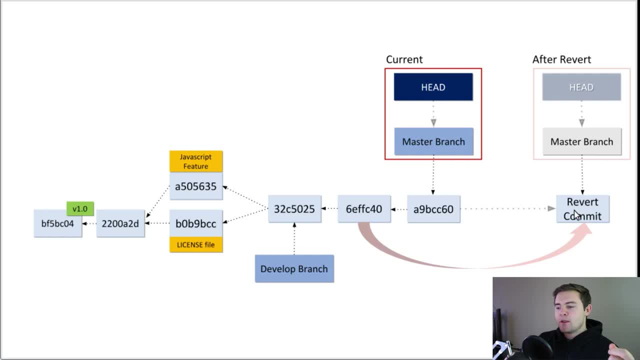 push them forward into a new commit that will reflect those changes. So, in effect, what's happening is we are effectively deleting- we're not really deleting, but we're deleting this A9B commit and we're going back to this 6EFF commit. 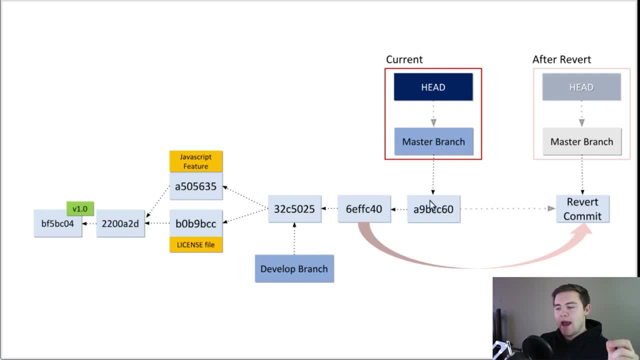 But all the while, we are keeping the history that we had previously. So if we really wanted to go back to this A9B commit after the revert, we definitely could, and so therefore we're not actually losing any of our files. So again, this is very useful if you're working on a team. 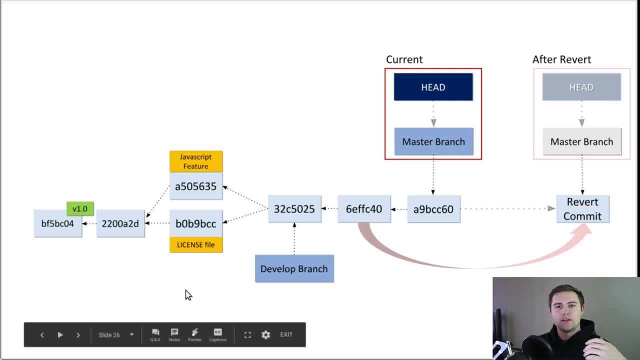 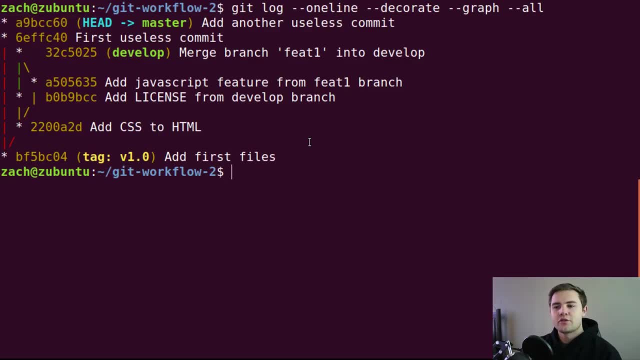 and you wanted to go back to a point in time without actually overwriting any of your team members' work For this command. we're going to go through two separate reversions. The first one is going to be a reversion to the most previous commit, and the second one is going to be 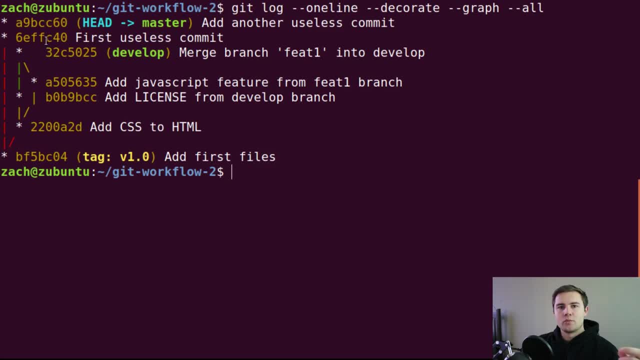 a reversion to this merge commit, which will be a little bit tricky because we have to take a few extra steps. So let's first start off with the easy reversion, and that is to the previous commit. The first thing we'll do is: 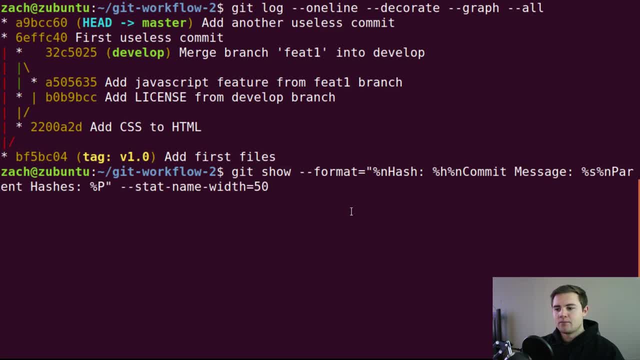 use this command. You can kind of copy what I've written here into your terminal. This is a command that I kind of formatted before I started the video so that we can see an individual commit a little bit cleaner. So in this case I want to see what was in commit 6effc4o. 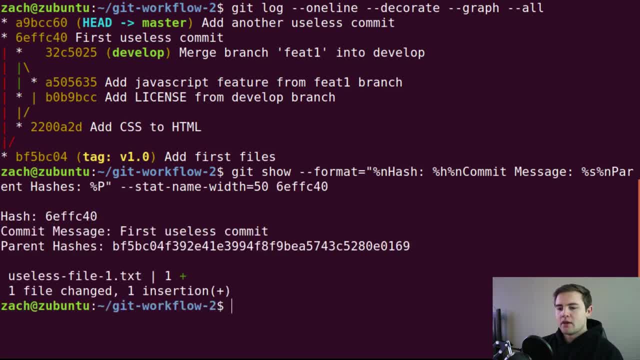 And when we press enter you'll see that we have a hash of 6eff. whatever, the commit message was the first useless commit and basically all I did was added this useless file 1.txt. So that's all that was happening in. 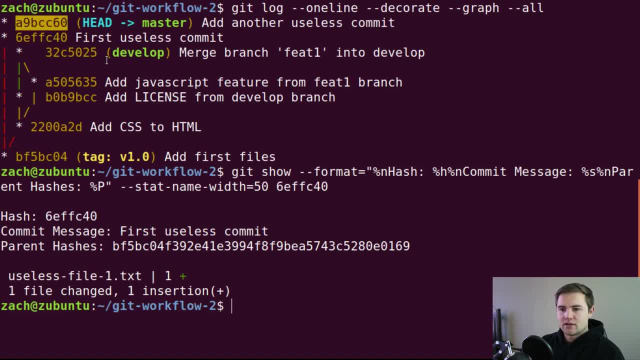 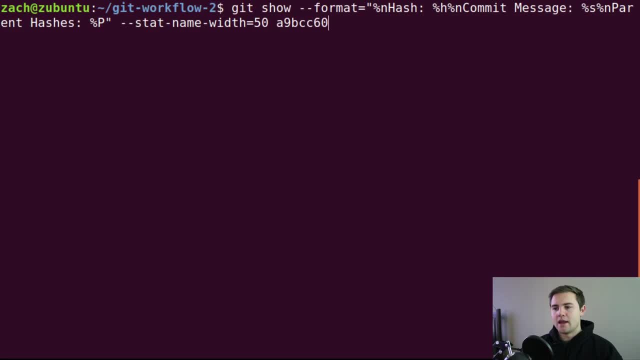 that commit and then we can also look at this most recent commit. So let me give us some room here and replace that commit hash, and now we can see that we added another useless commit and we added another useless file. So basically the effect of this first: 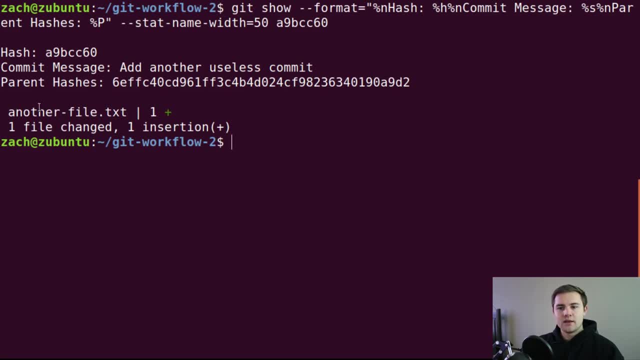 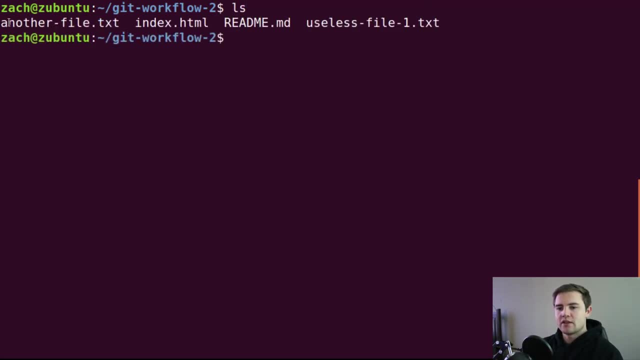 reversion is we're going to get rid of the most recent commit, and that would be another filetxt. If we print the contents of the working directory, you'll see that we have another filetxt. We can now revert back, so let me. 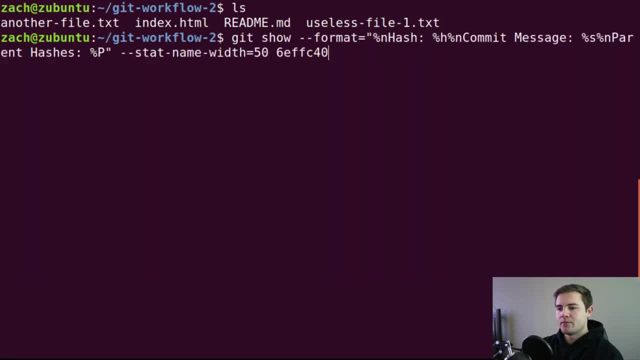 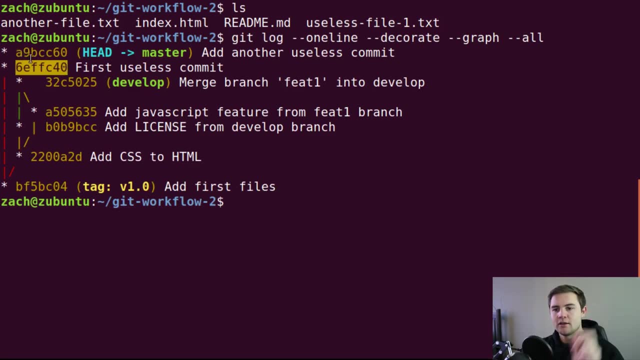 first show us the diagram of our repository. So we're going to revert back to this commit right here and effectively delete the a9b commit. To do that we'll type git revert head And what this represents. what head represents in this case? 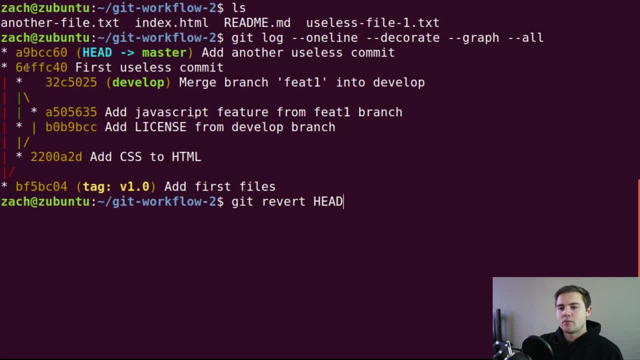 is the most recent commit, So that would be 6eff. We could also tack on a little tilde, which would be the second most recent commit. We could add another one for the third most recent commit, so on and so forth. 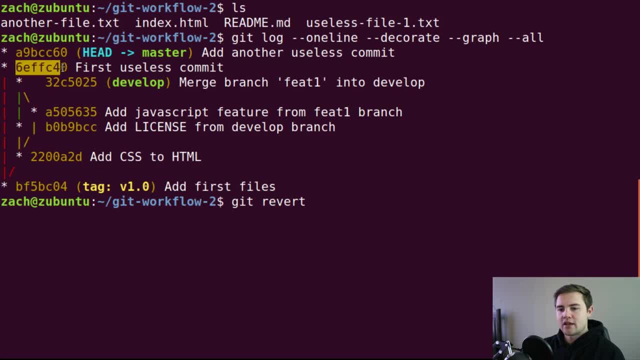 Another option we have is to just take the commit that we want to revert back to and enter that in there. So we'll use the first option. we'll just use head and when we press enter we're going to get a reversion message. we'll just 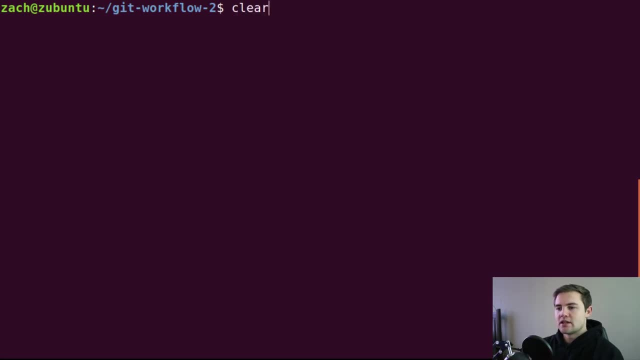 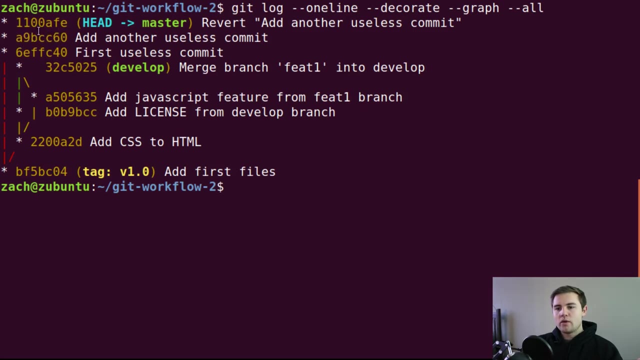 accept that and then you can now see that we have a little bit different repository. Previously we were right here, and now we've created an entirely brand new commit 1100, that has the snapshot of the files at the first useless commit. 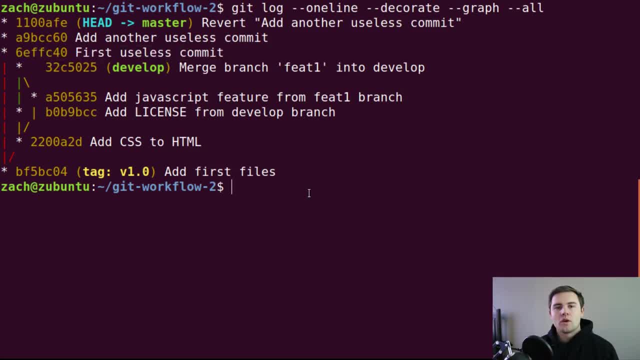 but it's pulled it forward in time. What I'm now going to do is run the git reset command. We haven't learned this yet, so don't worry about what this means. I'm basically just undoing what we just did with the revert, so I'm 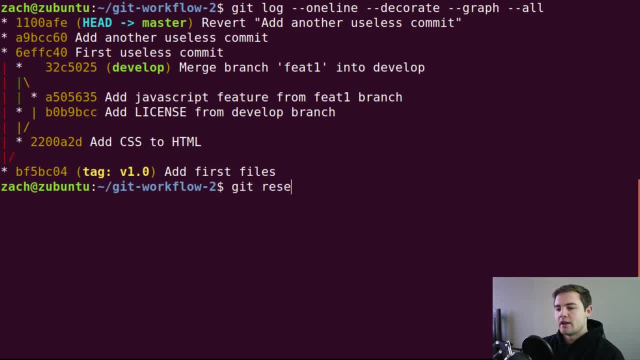 actually deleting that revert commit completely. The way that I do that is to git reset hard and then copy in this commit that we want to go back to. So I'll press enter and now, if we logged out, you see, we're back where we started. 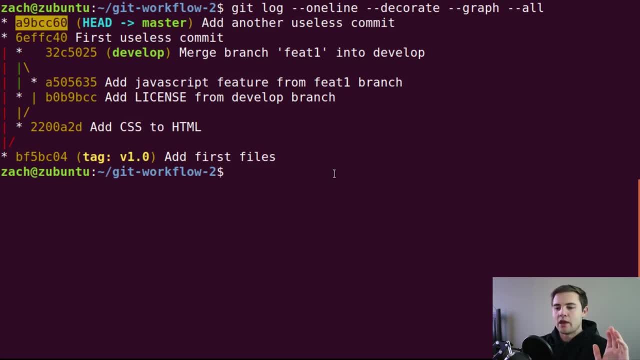 at another useless commit and we have no history of doing the reversion Once again. don't worry about that. I'll explain it in a few minutes. The second reversion that we're going to do is revert back to this develop branch. 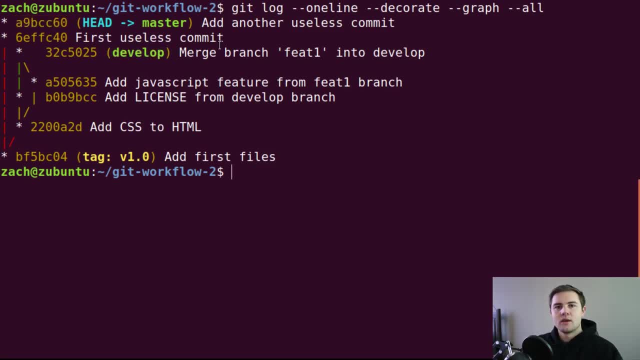 where we merged feature 1 into develop. So we've got these useless commits and we have no reason to keep them in the history of our repository. We basically just want to revert back to the develop and work from there The way that we do that. 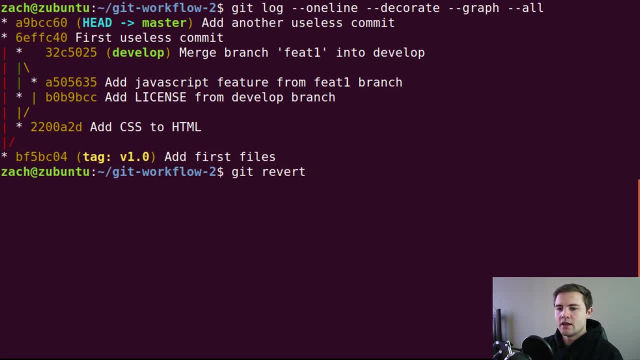 is. you would think just type git revert and then put in the hash of that commit, but it's going to say the revert has failed because we didn't specify something very important And that is what parent we want to actually revert from. So in other words, this merge commit. 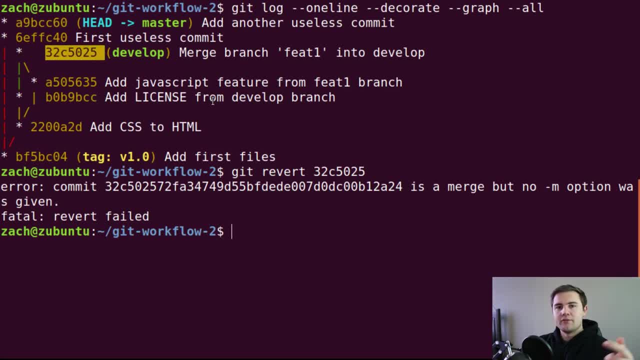 right here has two parents. It has the develop branch parent and the feature 1 branch parent, since what we are basically doing at that commit is taking two branches and merging them back together. So we have to choose which one of these parents that we want to revert back to and based on which one. 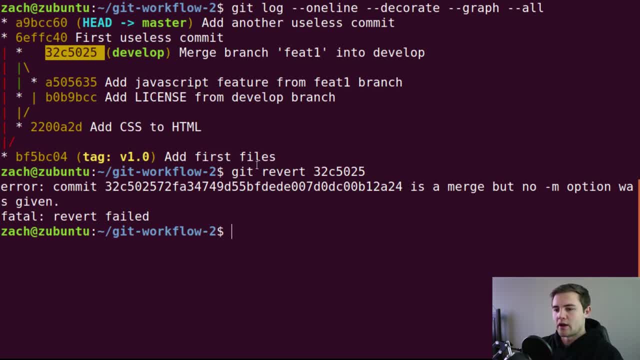 we choose. we'll see some different files in our working directory. To better see what was going on, let's first look at these two commits right here, the two that we actually merged together, and then we'll look at the actual merge commit to see. 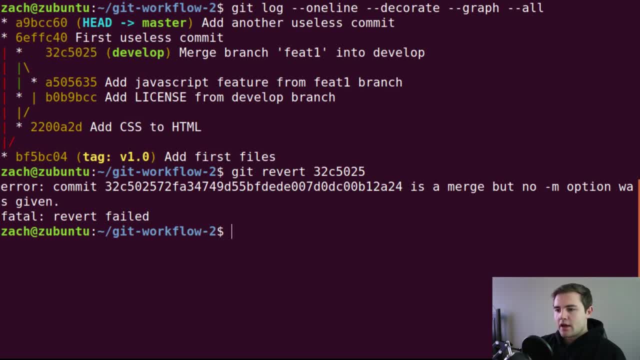 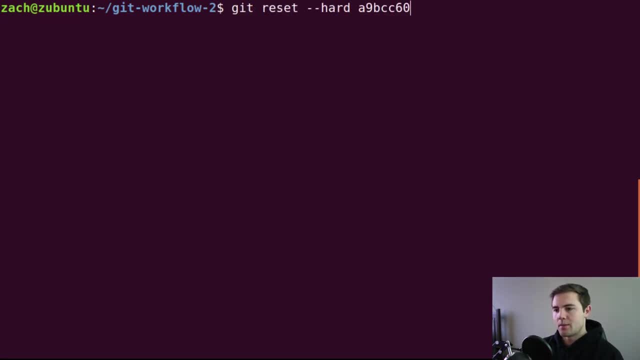 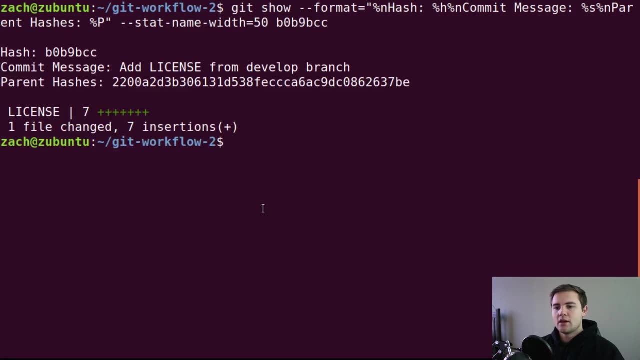 the two parents that we're dealing with. So again, we're going to start with this one and I'll use my pre-formatted command that we had typed in earlier. so right here, And I'll throw in that commit. You can see that the 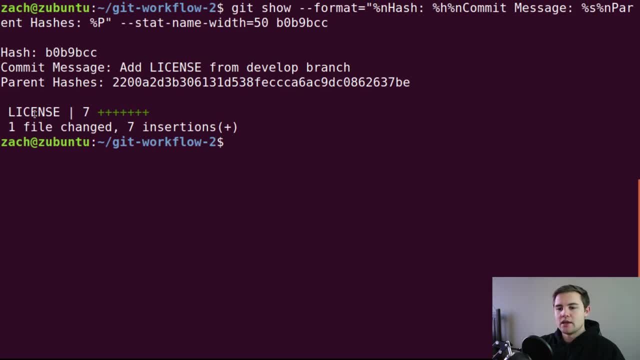 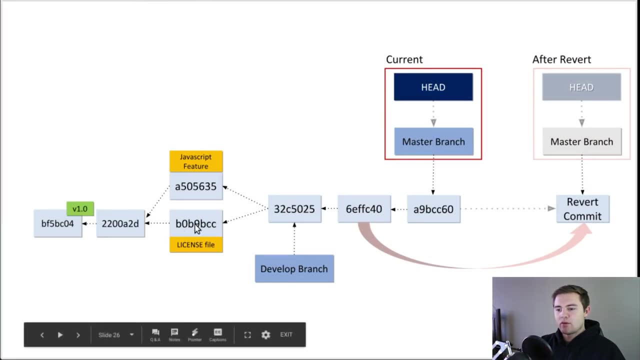 0b9bcc. hash is going to be the license edition. We can also see this in the diagram. So here's the license file that we committed, and then the JavaScript feature is the a505 commit. So we can also see that. Now let's take a look at this. 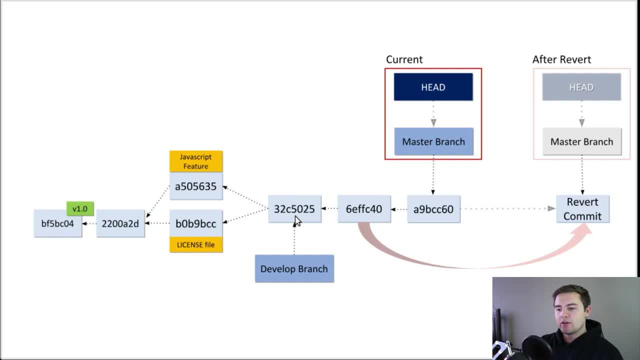 commit, where we actually merged it together and figure out what the index of each of these parents are, Because our goal here is to actually delete the JavaScript feature out of our repository. You know, maybe it didn't work, it kind of messed things up and we just don't want it anymore. So the way that 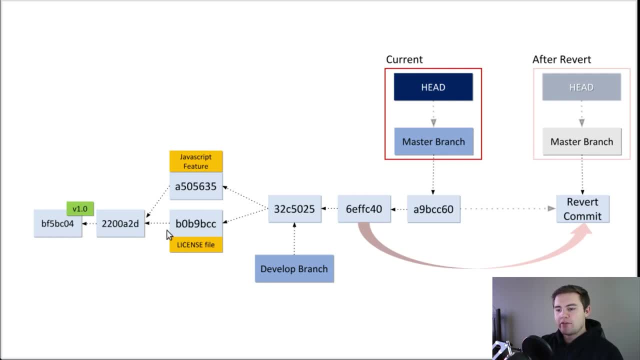 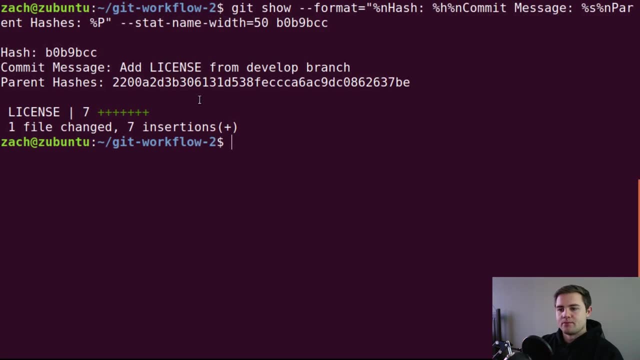 we'll do that is by specifying the develop branch, which had the license file in it, as the parent for this merge Or not the merge, the reversion. So in this case we need to copy the commit hash for the merge commit. 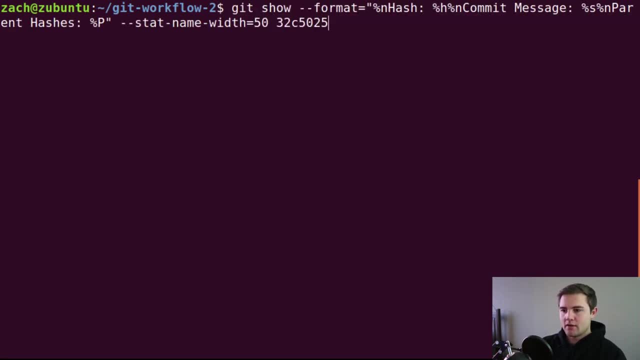 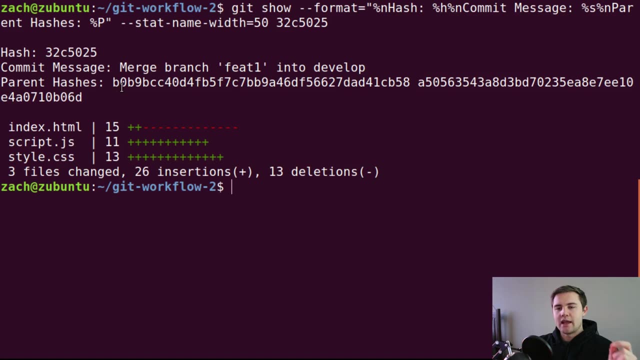 and plug that into our pre-formatted command And you'll see that we have two parent hashes And, reading left to right, we actually can add them together. So we have the index of this first one is 1, the index of the second one is 2.. And if you had maybe 3 or 4, 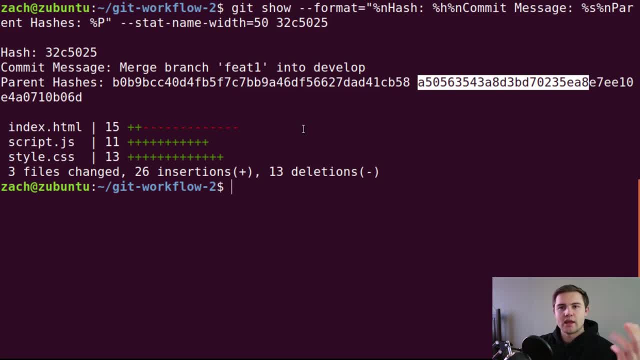 parents, which would be kind of unlikely. it would be 3 and 4.. Now you don't know what this means quite yet, but we'll use these indexes in the git revert commit itself. So let's remember, we have the bob one which is going to be: 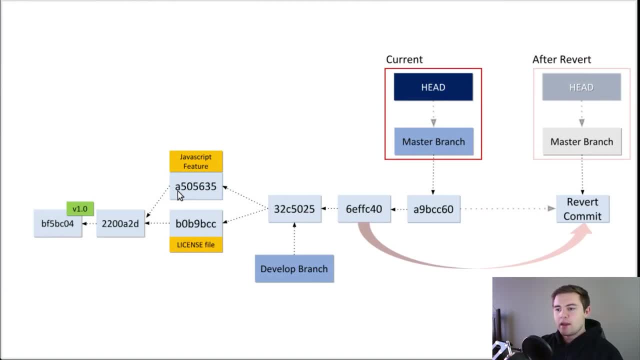 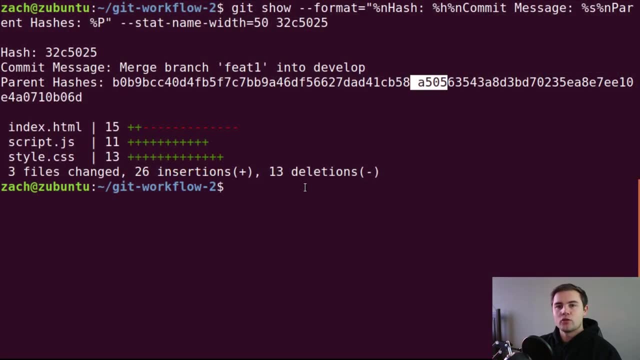 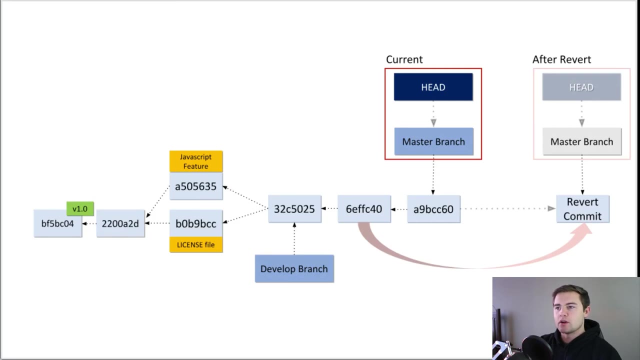 the license file or the develop branch, And then you have the- let's see the a505, which would be index number 2. And that was the JavaScript feature. So we don't really want to include that. So in other words, 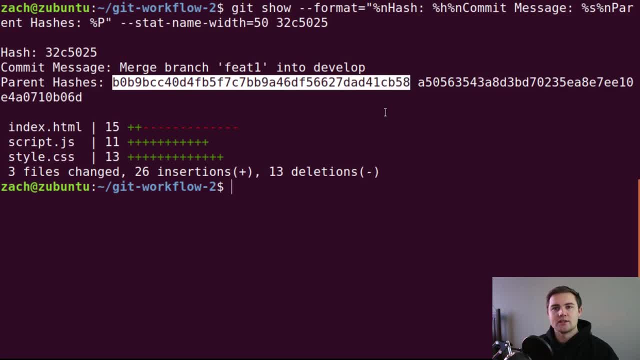 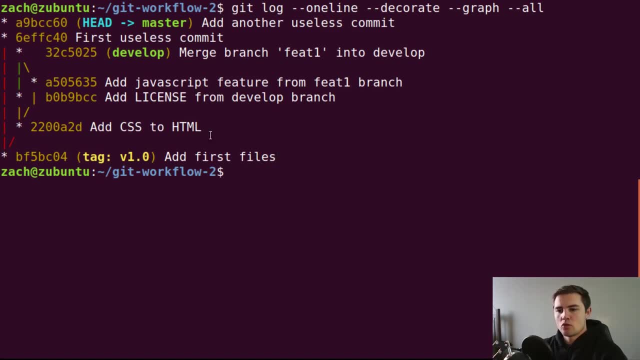 we're going to use the first parent hash, which is represented by index number 1.. We're about ready to do this reversion. Let's look at our repo one more time. Remember, we're going to go back to this commit right here. That's the one we want to revert back to. 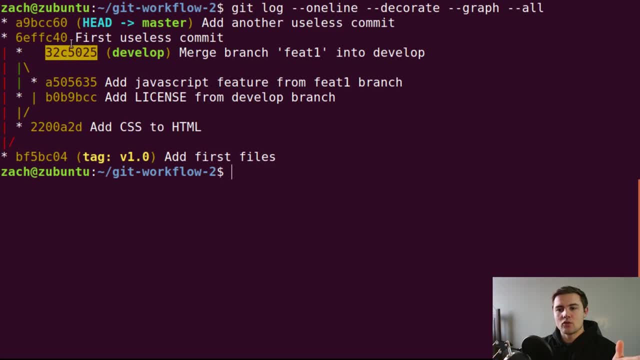 And remember, we're not deleting anything here. we're just taking the snapshot at this given point in time and creating a new commit that reflects that. The tricky part is we need to tell git which parent to use, And we had derived that we want the develop branch and 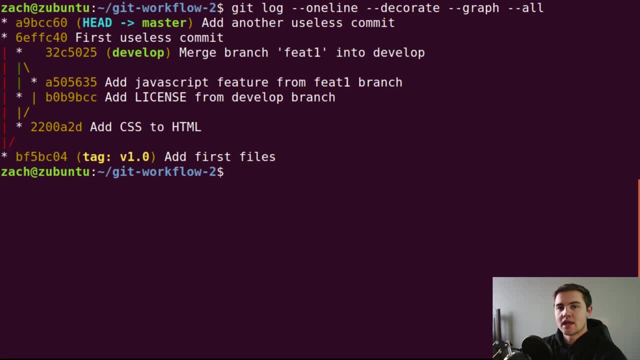 that is going to be index number 1.. We'll say git revert, and then this is where we pass in the index. so to the main line: Basically tells it what parent to use And then finally you'll plug in the commit that you want to revert. 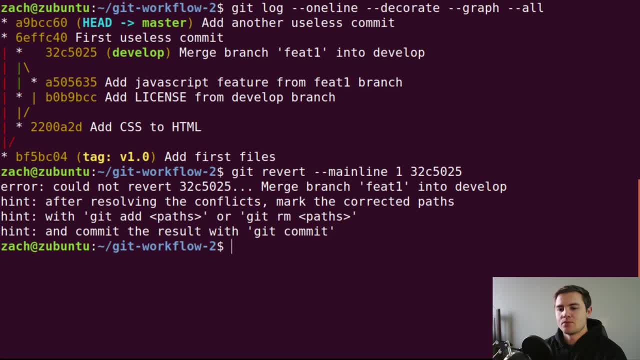 to And you're going to see this nasty commit message. The reason being is because we have a merge conflict due to the fact that we had edited the indexhtml file in both the develop branch and the feature 1 branch before that commit. We need to resolve that really quickly. All we need to 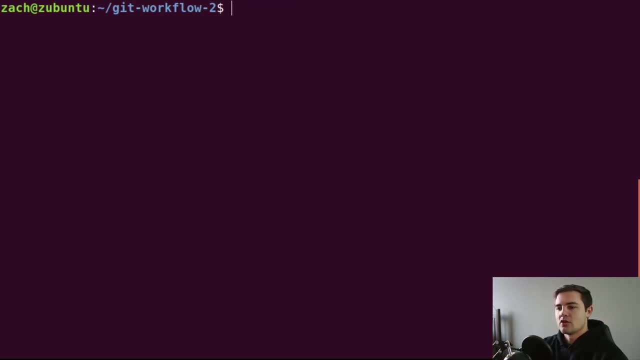 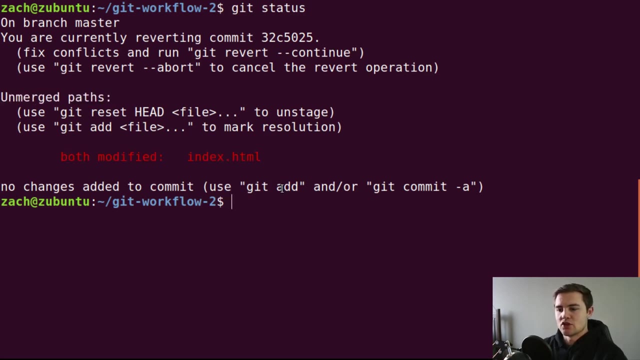 do is open up vim with the problem file and you can see that it tells us right here with git status that we have an unmerged path for the indexhtml. So that's where I'm getting that And we need to go into vim edit. 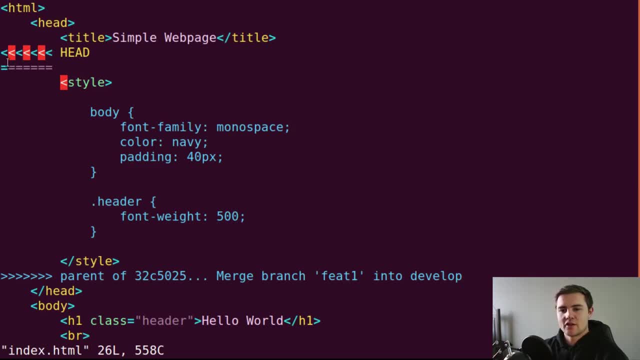 that You'll see that the conflict is highlighted here with these two lines and then finally this one. It says the merge branch feature 1 into develop. That's where this conflict is coming from And basically you don't need to really worry about. 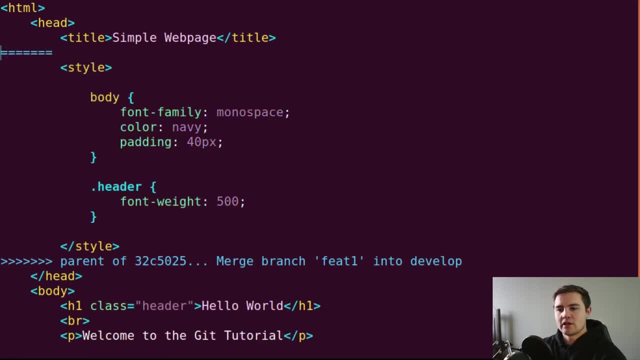 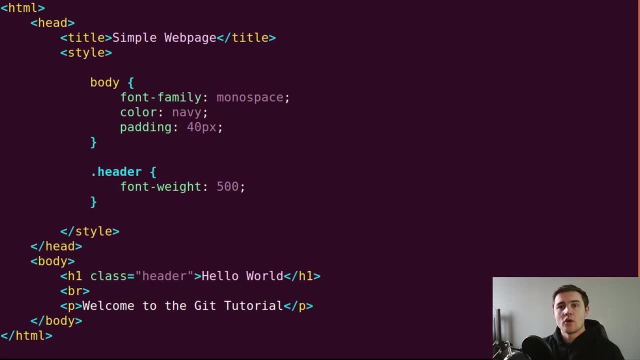 what we're going to keep. We just need to fix it. So let's just delete these right here. And this is going to be the new state of our indexhtml file, which was the same state that we had prior to creating the feature branch. So we'll. 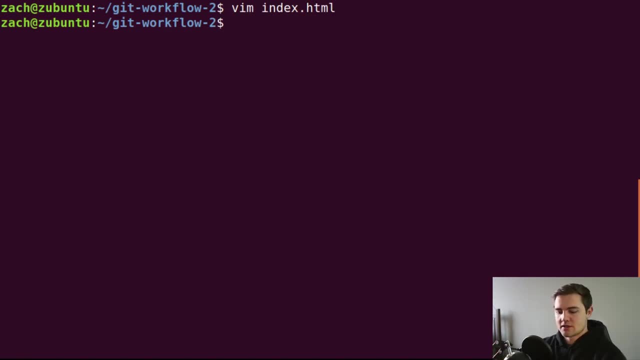 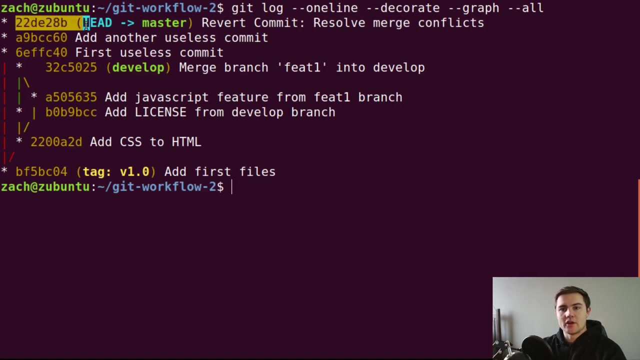 save and quit. We have resolved those conflicts. So now we can add indexhtml and commit it. So we'll say revert, commit, resolve, merge conflicts. And we can now see what the repository looks like And you'll see that we have this new commit here which represents the state of the repository. 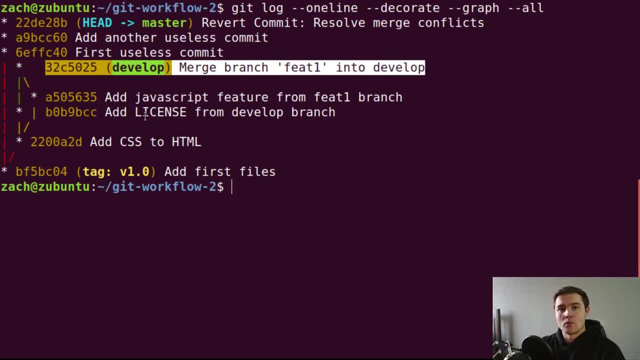 back at this commit without the feature 1 branch integrated into it. So in other words, we have this brand new state of the repository while also keeping all the history of the repository. So this would be great if you actually had a feature that may have broken the repository, but you 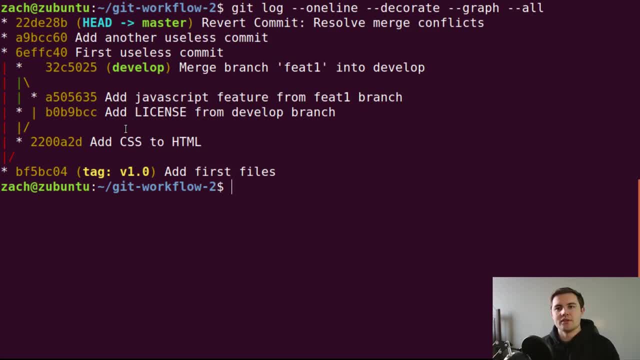 don't want to completely delete it, in case someone was going to use it in the future, Maybe reference back to it for learning purposes, I don't know. So that's the effectiveness of the git revert command. I know it's a little bit complex. 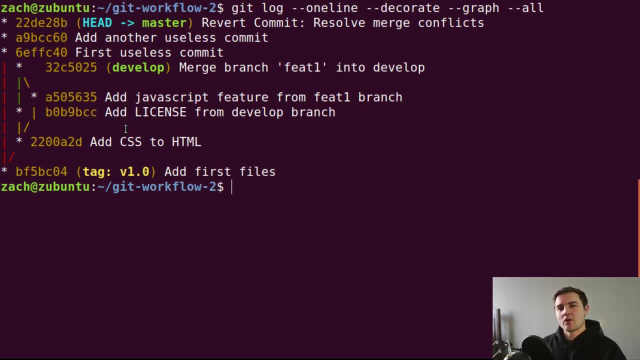 for this second example. but many times you're not going to have to deal with reverting back to a merge commit. I just wanted to show it to you in case that maybe you ran into that situation and you were like: what do I do So? hopefully that clears some. 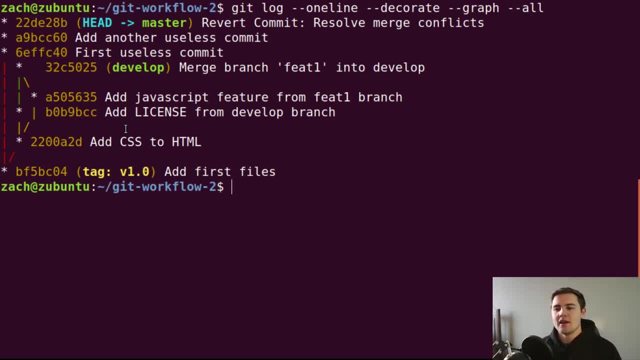 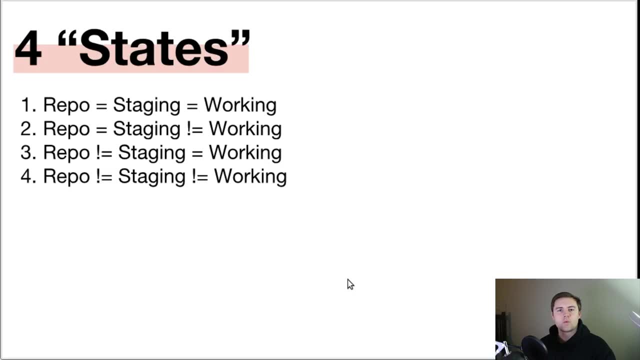 things up and you won't be so nervous when it throws these nasty messages back at you when you try to revert. There's one more command that we'll look at, which is the git reset command. We'll do a quick review here, because I think we've learned quite a lot in the last few. 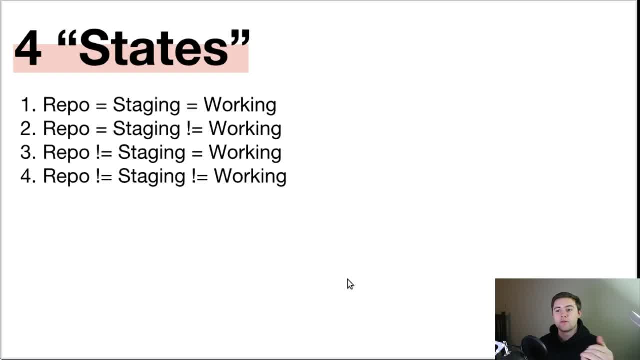 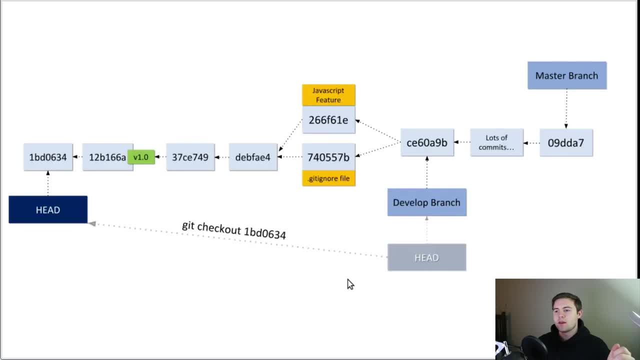 minutes. First, just a quick review of the four states. Gotta always keep that in mind because it's going to affect all three of these commands. So we first looked at the git checkout command, which essentially takes the head pointer and moves the head pointer to a different spot in the repository. 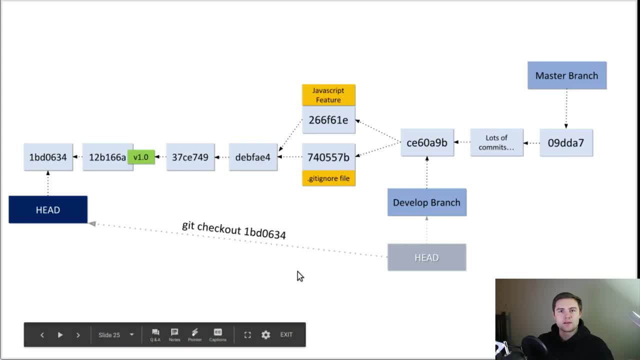 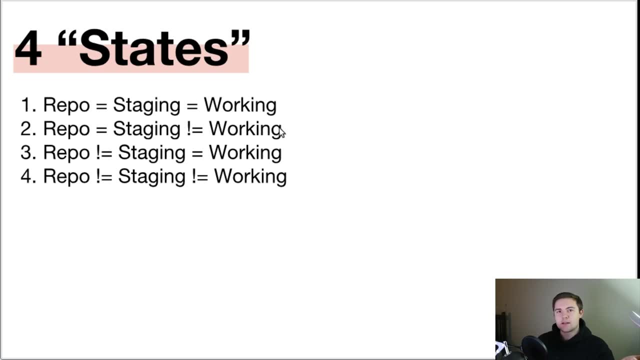 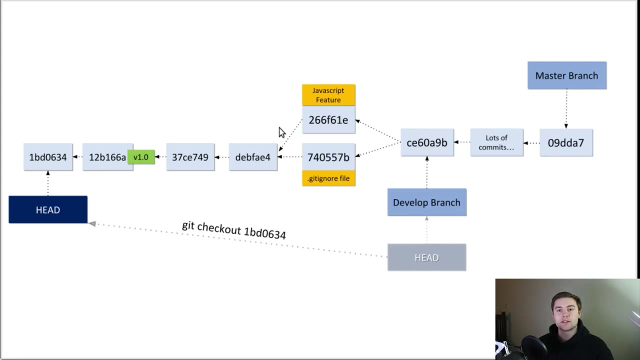 This could either be a branch or an individual commit, And in order to do a git checkout, you'll need to be in state number one. If you're not in state number one, then it will ask you to either commit or stash your changes. We looked at how to stash changes, so you should. 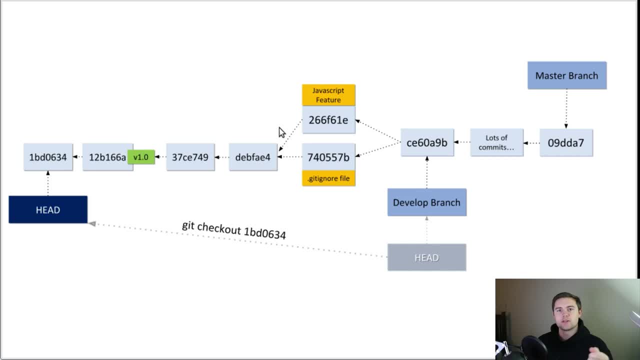 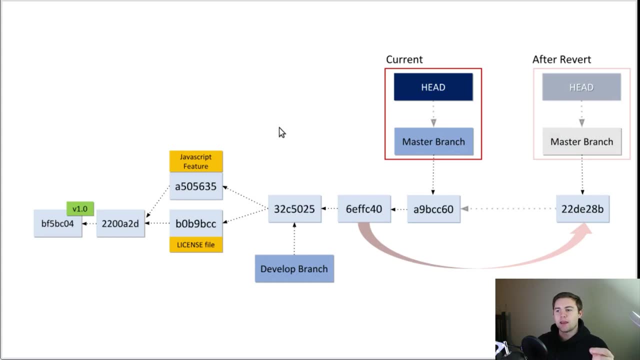 be able to handle that. Nevertheless, always make sure you're in state number one before performing a git checkout. We also looked at a git reversion, And we saw two examples of that. The first one was pretty simple- We just reverted back to the most previous commit- While the second one was a little bit more. 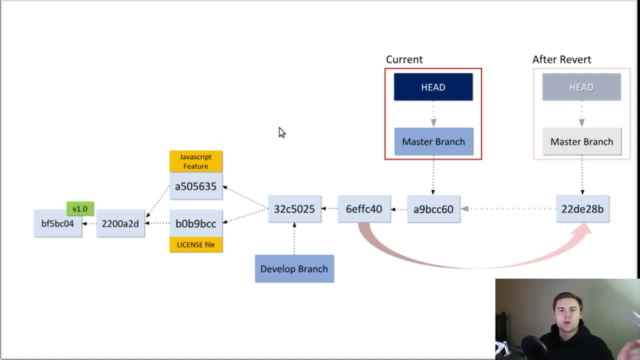 complex where we reverted back to a merge commit. Now, remember, with this revert command, what we're doing is we are going back to a point in time, so say the 6eff commit, and we're taking the snapshot of the files at that commit. 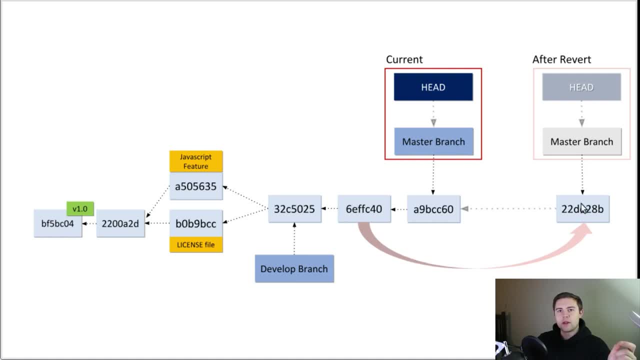 and pulling those forward and replacing what is currently at the a9 bcc 6o commit, which is where the head and the master branch are pointing at the moment. So, in effect, we move forward one commit in the repository, except we now are. 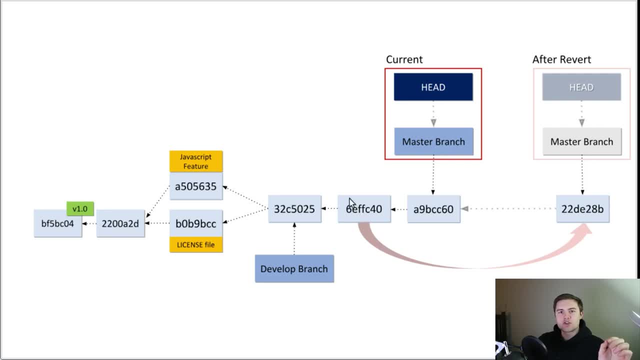 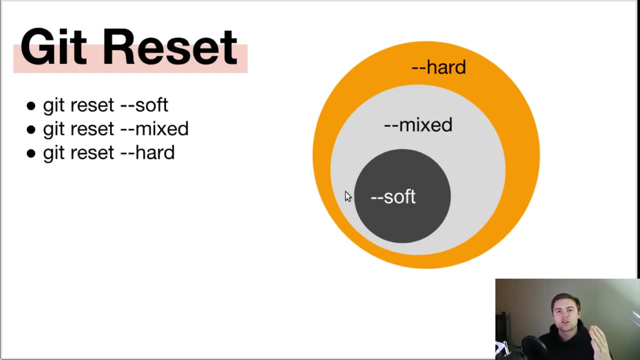 back at a previous state. We still have the history of everything that we've done. Now, with the git reset command, we're going to be actually rewriting history. in a sense, We're going to be completely deleting some of the commits that we have made and depending 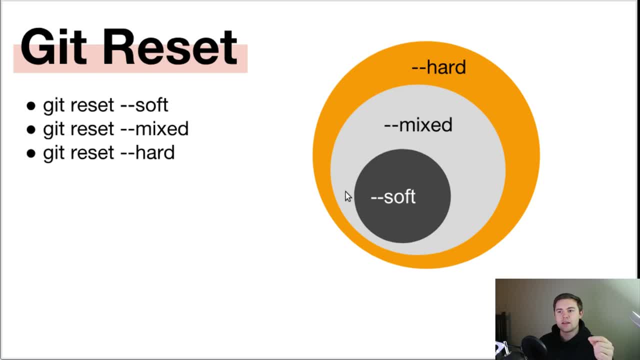 on how you use it, you're going to have a slightly more dramatic effect. So I've put this git reset command out in this little circle matrix- whatever you want to call it- because each of the commands, each of the versions of the git reset command are going to. 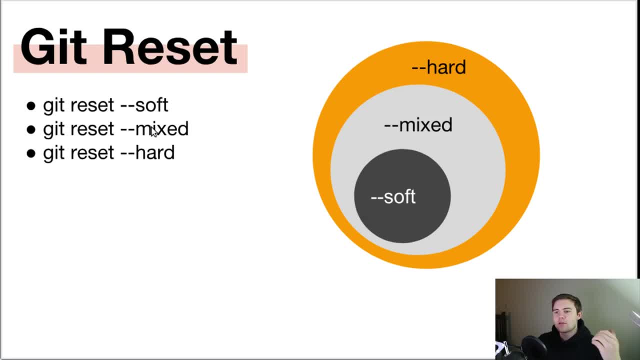 successively do a little bit more. So in other words, if you ran the git reset hard command, that's going to run the git reset soft, the git reset mixed and finally the git reset hard command all in one If you do just the git reset. 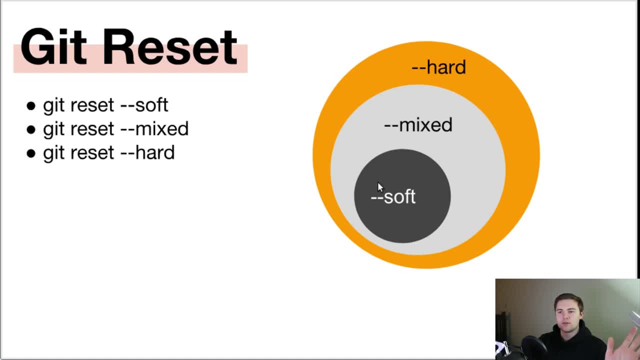 soft. it'll only do the reset soft. It won't do anything with the mixed or hard. So that's kind of how you should visualize this particular command. There's basically three different versions that you can use. Now we're going to start with the git reset soft, but 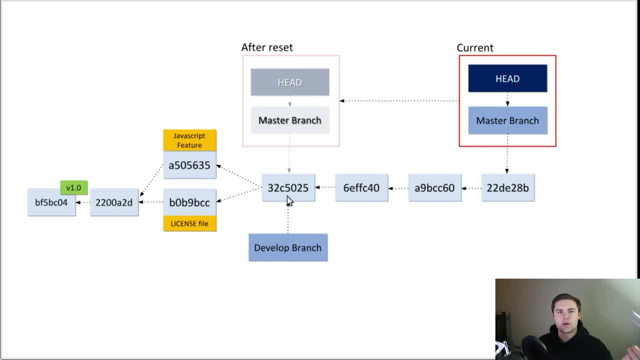 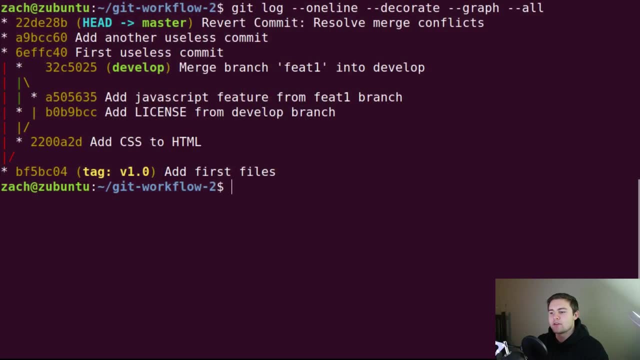 before doing so, we'll take a look at what this is going to do to our repository. So currently, this is what our repository looks like. You can see that back in the terminal with the git log command, but this is a little bit more visual for you. 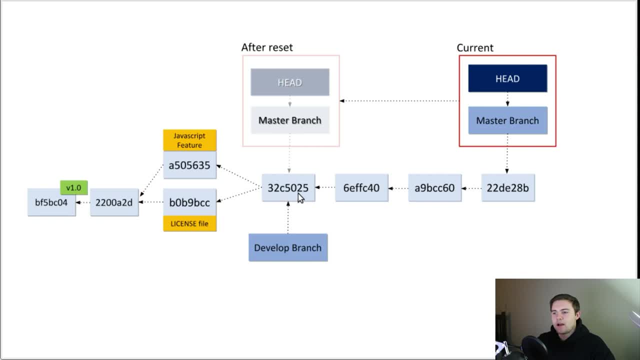 And currently we are sitting at the 32c5025 with the develop branch and 22de28b with the master branch and the head pointer, which basically means that that's where if we made changes to any files, that's where they would go right there. Now the reset command. 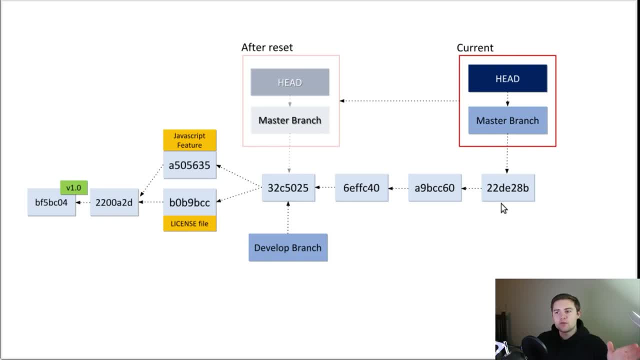 no matter what version of it you use, it's going to have the effect of moving both the head and the branch that the head points at back in time to a specific commit. In this case, I've shown an example where maybe we wanted to. 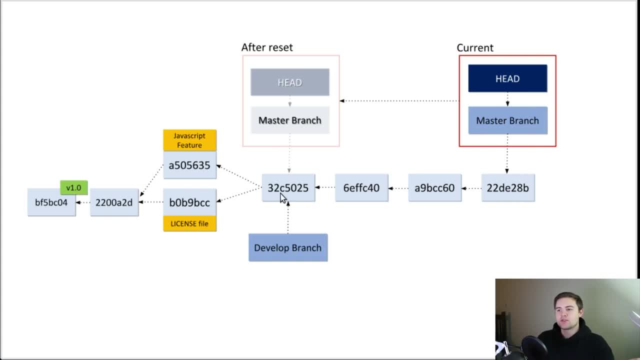 reset back to the commit 32c5025.. And remember this one right here: the 22de is our revert commit And if we reset back to 32c5, that's actually going to reset it so much that we have. 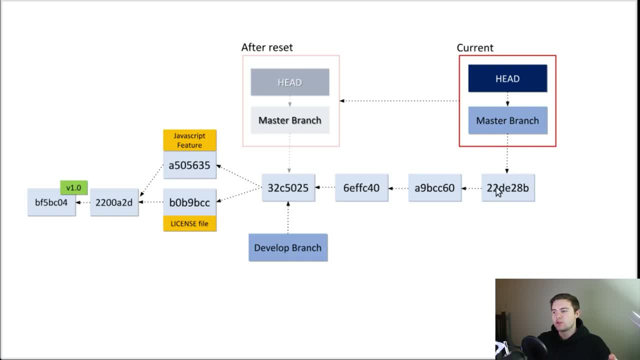 the JavaScript feature back in our repo. Remember the 22d commit- that's the revert commit- kind of took out the feature 1 where we added that JavaScript. but since that is only a reversion and we just basically took the state back here and pulled it, 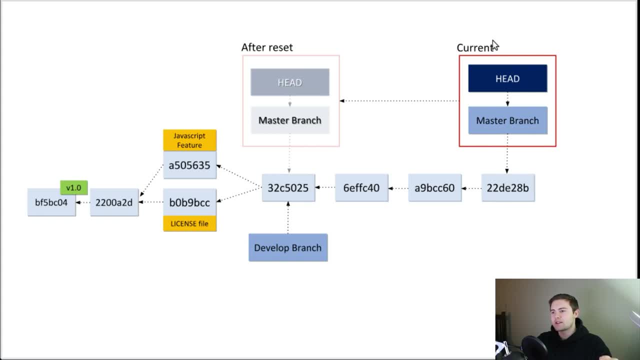 forward. if we reset and moved all of this stuff back here, we're going to have that feature 1 branch integrated into our repository again. In effect, these three commits right here, the 60f, a9b and 22d. they're. 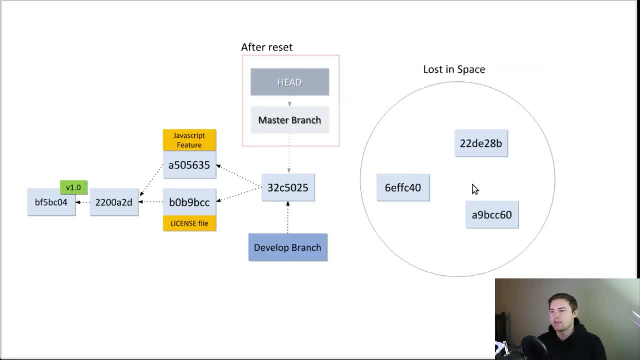 all going to just kind of float in space, And you'll see that once we have reset we're going to have these commits somewhere out in space, but we have no way of referring to them and therefore this command can actually get a little bit dangerous, because 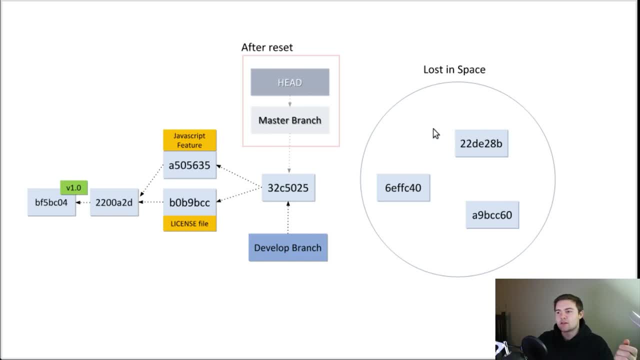 if you reset back to a place and then realize, oh wait, I wanted to go back, you can't really do so Now. depending on which version of the command that you use, you may or may not delete the working directory. So in other words, 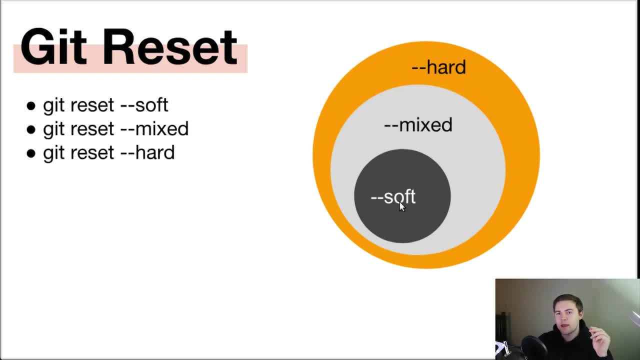 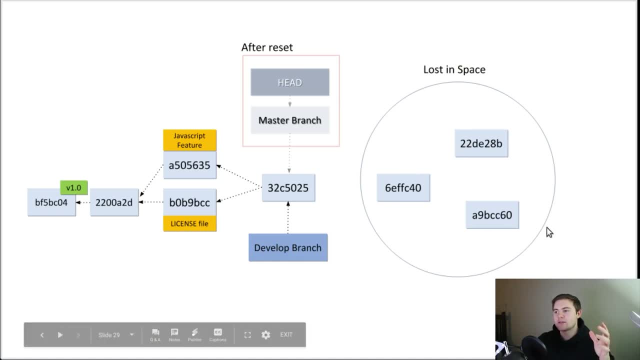 if we use the git reset soft command and then we come back to this state, we will still have the file changes that went into these commits. they'll just all be globbed together. Now, if we use the git reset hard version, we're going to basically delete. 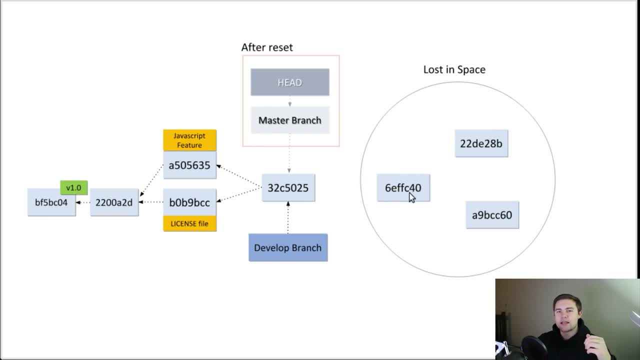 everything out here. So anything that was added or removed or modified in any of these three commits out here we're not going to have any recollection of and we'll have zero way of getting those back. So you do have to be careful with. 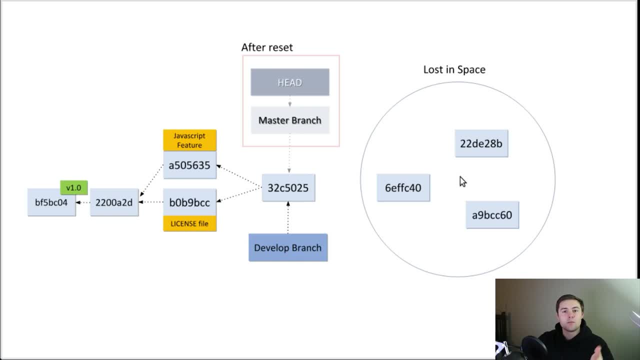 the git reset hard command and even the soft and mixed commands. Alright, enough explanation, let's get into actually writing some of the commands. As we run the three different versions of the git reset command, be aware of what state it puts us in. So at the moment, 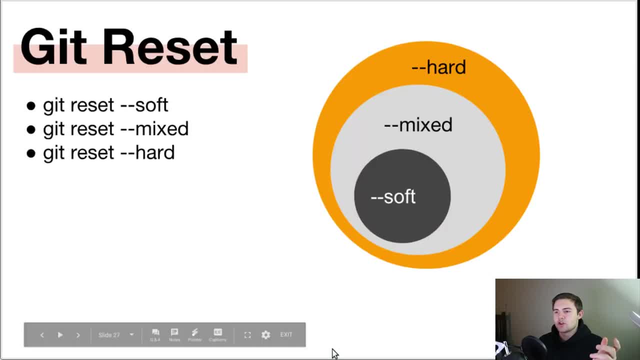 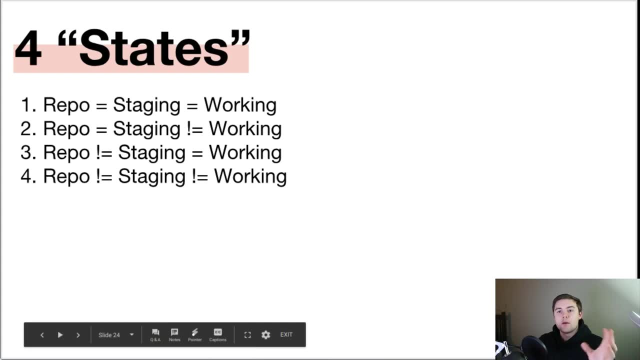 we are in state number one, or at least we should be. I'll put this up on the screen for reference. We're in state number one, where everything is synced up, But we'll keep a tab on which state we are moving to with each version. 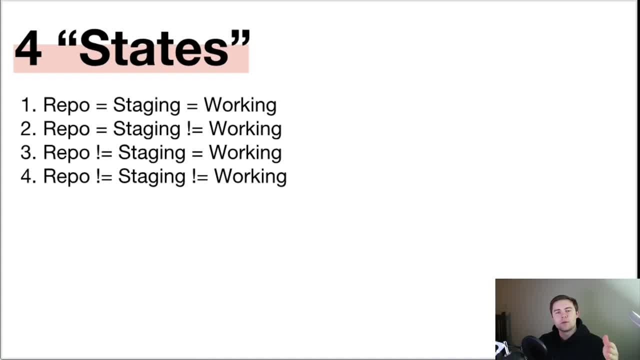 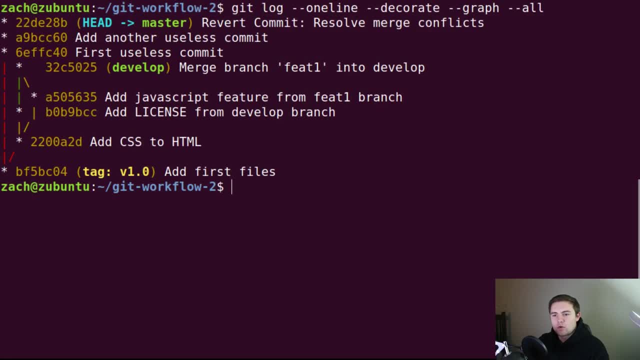 of the git reset command, because that is ultimately the difference between each of the three. So let me get back to the terminal. This is what our repository looks like right now And, given the fact that this command is pretty much permanent, we're not going to be too aggressive here. I only 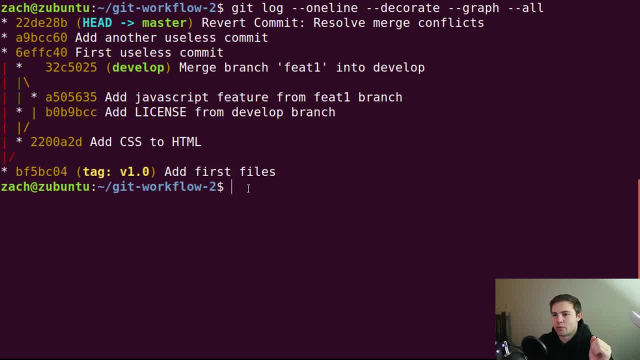 get one take with this, otherwise we have to redo the whole repository. So for this first reset, what we're going to do is essentially delete this reversion that we just did. So in other words, we want to reset back to the A9BCC60. 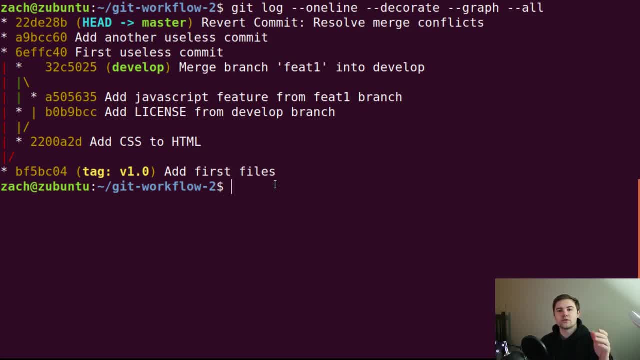 commit And therefore when we do that, we're going to. if you remember, the revert commit basically took out feature one and therefore it took out the JavaScript files. So if we type ls, you're not going to see any sort of JavaScript here, And if we 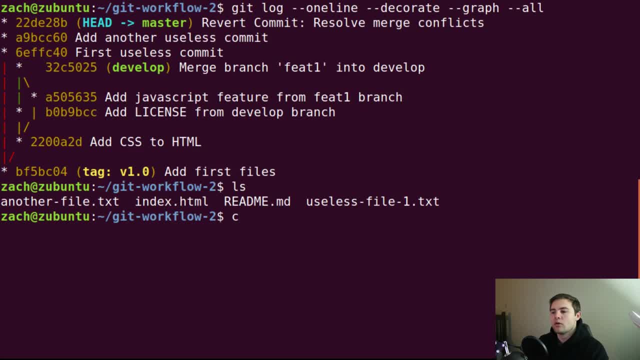 remove that, revert, commit or reset it. we should see all the feature one files. So let's do that right now. Reset and then soft. Make sure that you add the soft flag in. If you don't add a flag, it'll just default to. 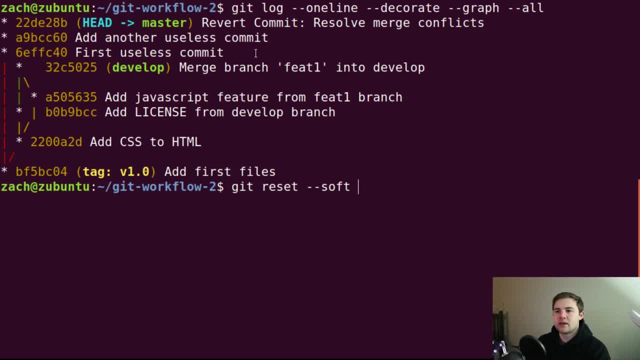 the mixed version And then, finally, we will enter the commit that we want to go back to. So we are going to move the head and the master branch back to A9BCC60 with this command And if we log out this repository again. 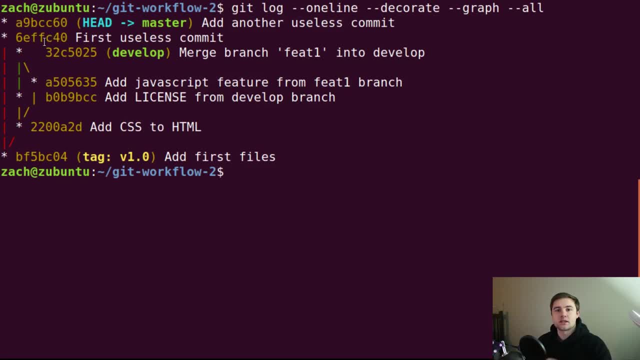 you'll see that that revert commit that was at the top is completely gone. We have no recollection of that happening except for the staging area. So it'll show you that in the staging area we have a modified file And that is going to. 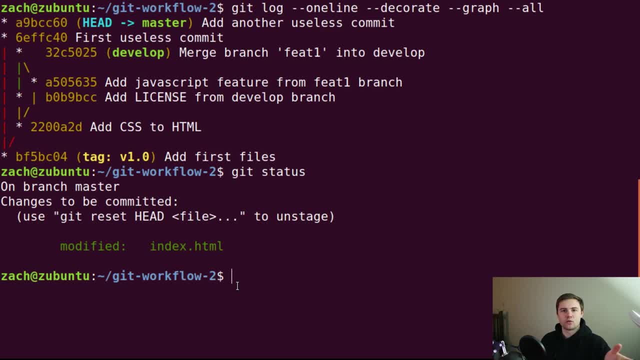 be the changes that were made from that given revert commit. So, if you remember, we kind of fixed the merge conflicts in the indexhtml. So that is going to be in the staging area after a git reset soft command. Now let's remember what state we are currently in. We should 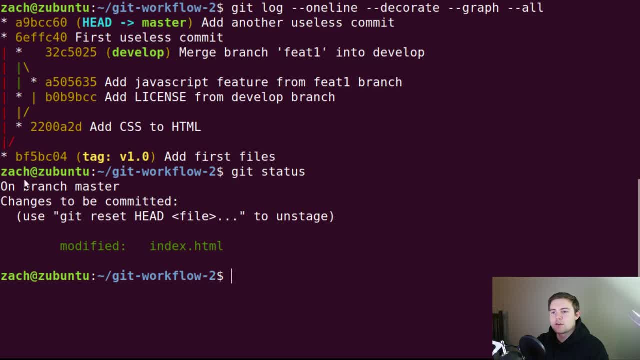 be in state number three, which is basically the repository, is not going to equal either the staging or working directory, but the staging area and the working directory are going to be equal. So that is what state we are in right now And if we wanted to, we could commit. 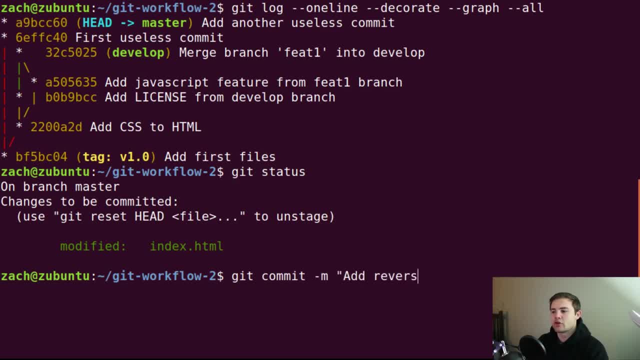 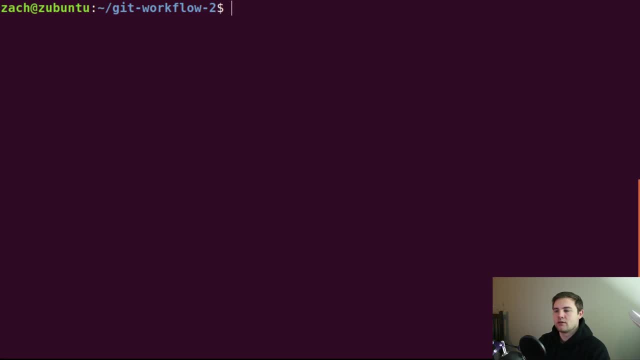 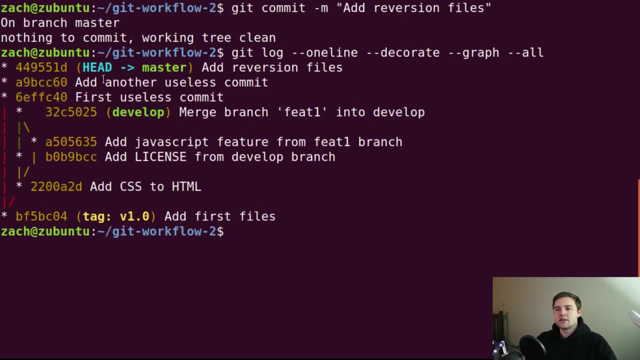 and say: add reversion files, And then basically what's going to happen here? when we log out the repository, that's not the log command There we go Is this is basically going to give us back our reversion, but it'll just have a different name. So, as you see, 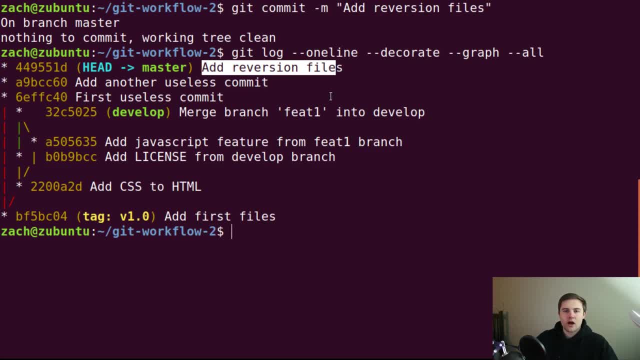 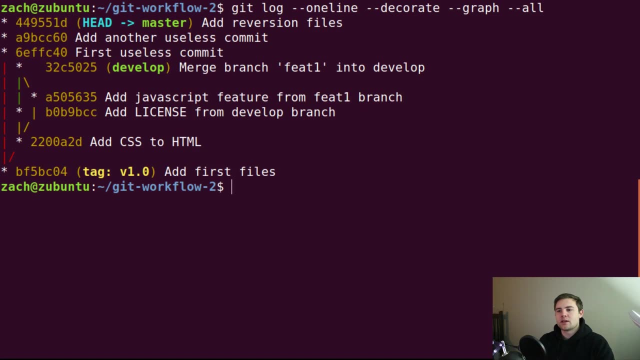 with the git reset soft command we can recover the files that we kind of reset, but we can never get the exact commits that we had previously back. The same goes for the git reset mixed command, Except this time instead of moving the head and whatever branch that 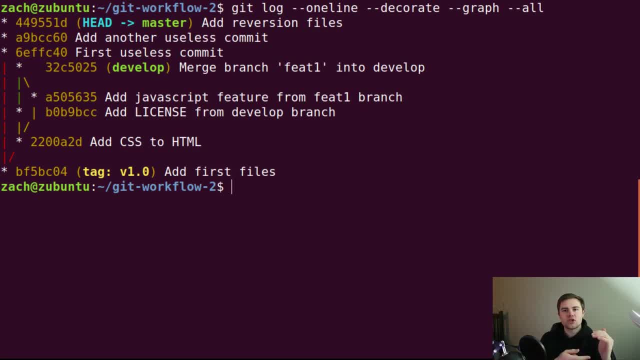 points to back to a given commit and then staging the working directory in the staging area. what it's going to do is move it back and just leave the working directory. It's not going to add anything to the staging area. So we can do that real quick. We can just type git reset. 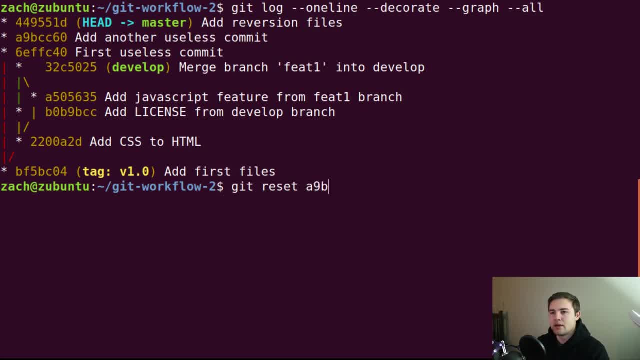 and then we'll go back to the A9 BCC 6.0 commit And notice I'm not putting in any flags here, because the mixed option is the default git reset option And when we reset it's going to say unstaged changes after. 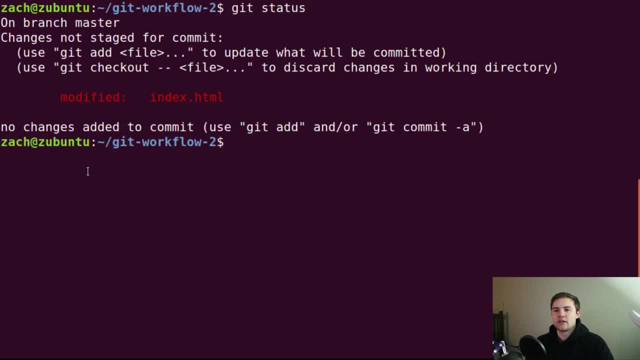 the reset And if we type git status, you'll see that we have changes not staged for commit. the indexhtml- And, if you remember, the changes not staged for commit- just represents the working directory and therefore this state would be, I believe, number 4.. So let's go. 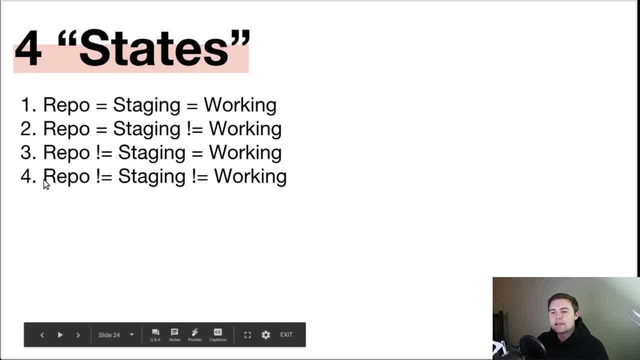 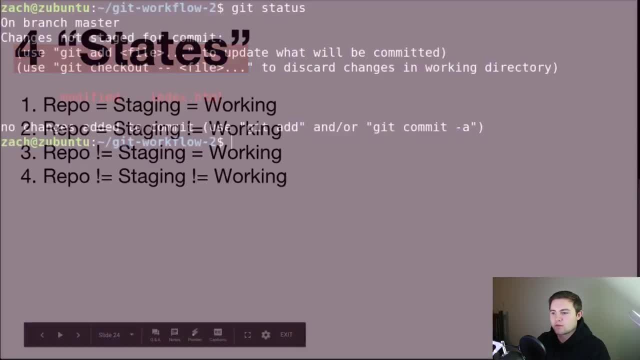 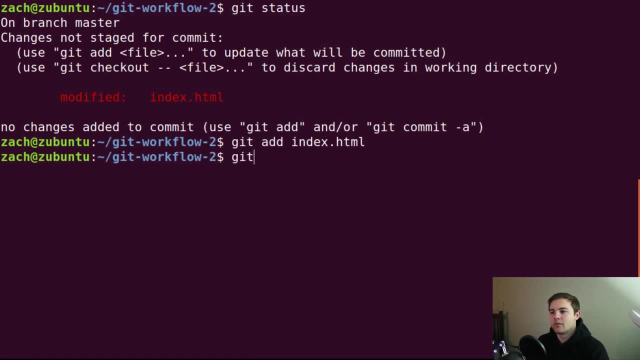 back to our PowerPoint, and we are indeed in state number 4.. The repository does not equal the staging area, which does not equal the working directory. Alright, so again, we can just add the indexhtml and recover the reversion once again. In this case we have the same exact. 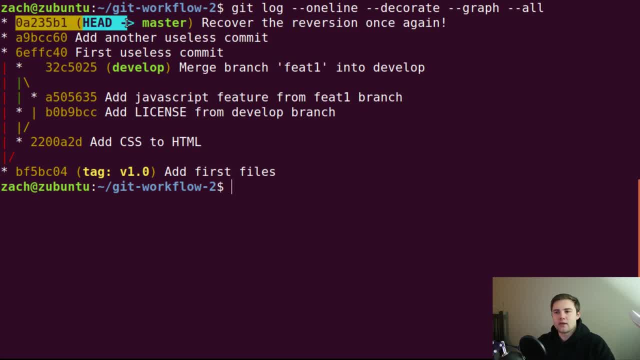 effect and when we look at our repository again, we have this commit that, basically, is recovering the reversion. Now, if we use the reset hard command, what it will do is it will move the head and whatever that points to, whatever branch that points to, back to a given. 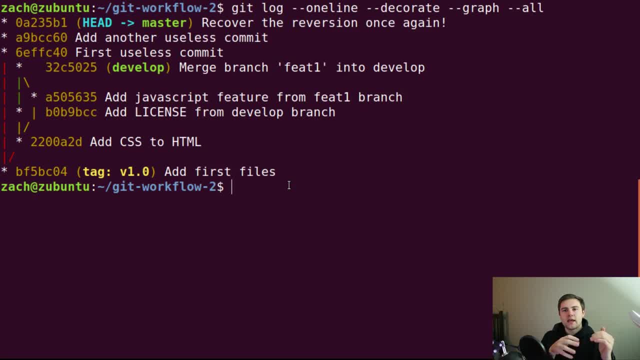 commit. It will then take all of the changes since that commit and delete them from the working directory, the staging area and the repository. So in other words, we have no way to get them back. So let's run that real quick, git reset hard, and then we will. 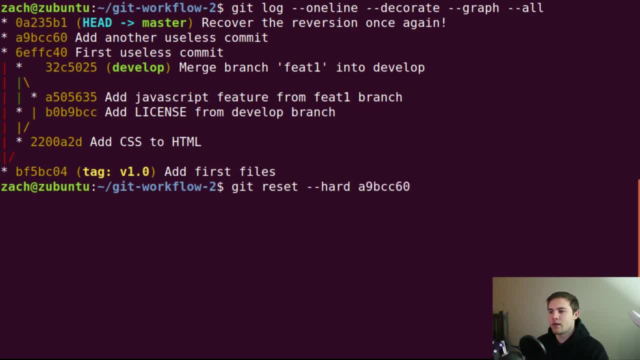 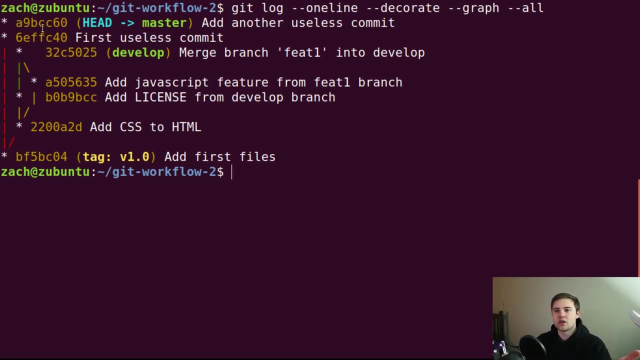 again go back to the A9BCC6O and right now we have no way of recovering that indexhtml or whatever we changed about it. And if we log out the repository you'll see that we pretty much don't have any recollection of the reversion. 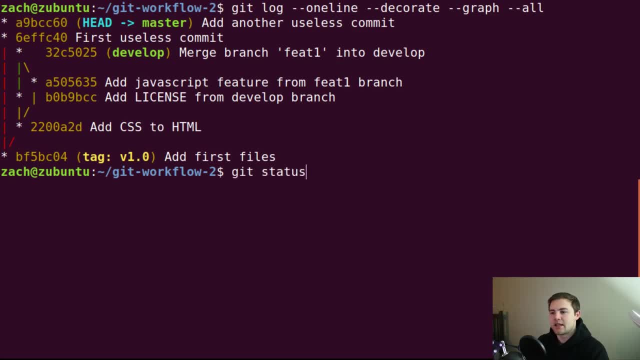 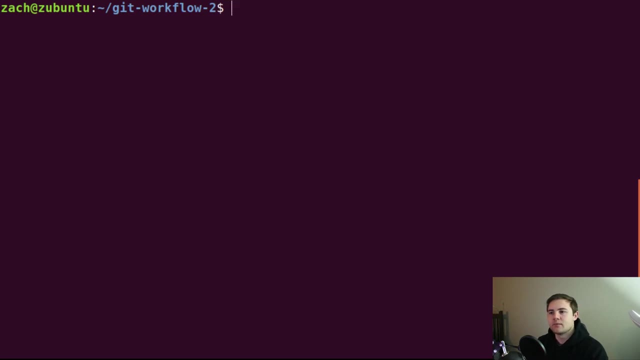 that we did earlier, And if we type git status, it should be in state number 1, where everything is synced up. So that is the effect of the git reset hard command, and you'll actually see this. so say we. maybe we will just add a. 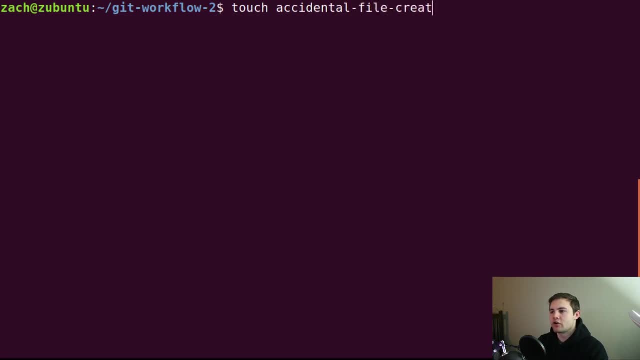 file here, so accidental file creation txt. Maybe this was a file that we didn't mean to add in there. it just got copied into our repository And when we say git status, it will of course pick up on this. it will figure out that there's something out there that we haven't quite. 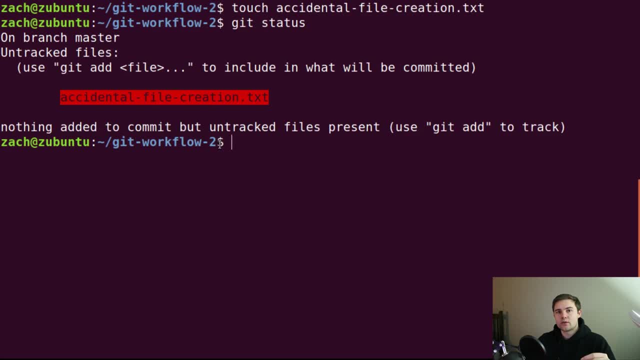 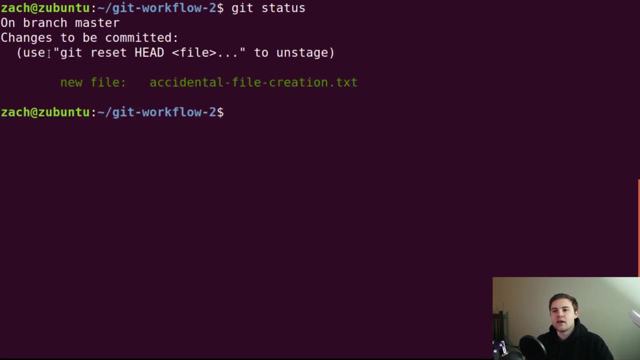 added to the staging area yet, So it's in our working directory but not the staging area. And then it will basically say: you need to add it, so we'll add that. and then when we type git status again, it will say: you can use the git reset head. 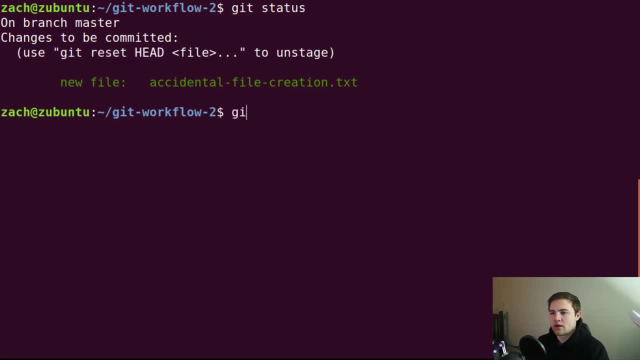 to unstage that, And so we could run git reset head to effectively use the git reset mixed command and go back to the most previous commit or the commit that we're basically on, and that will, in effect, throw this file back in the working directory. 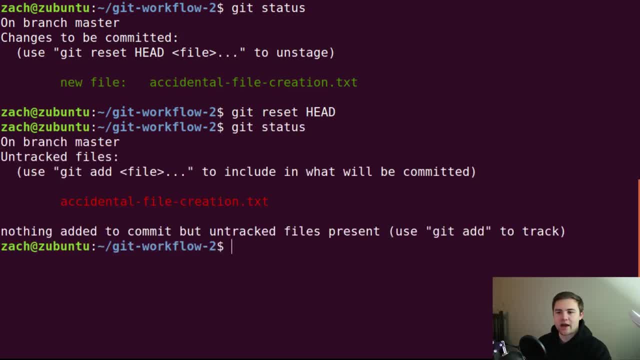 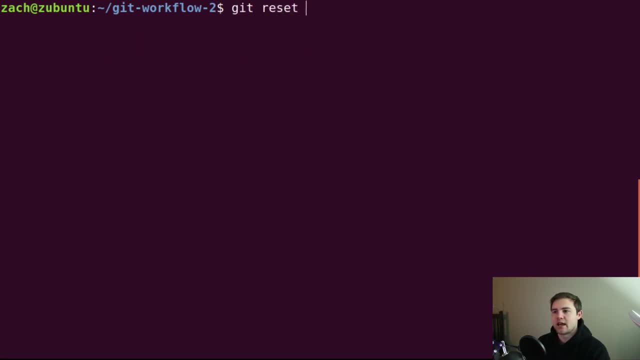 so again we run git status, it's back to our working directory. Let's just add it back one more time. and then this time, if we run git reset hard head, then we are going to delete that file entirely. and when we type git status, everything is clean. 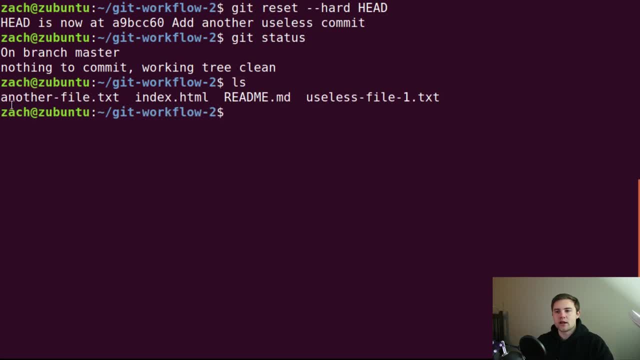 and when we print the contents of this directory, you won't see that file any longer. So that would be probably the most practical use of the git reset command is when you're just, like you know, want to kind of go back just a few steps. 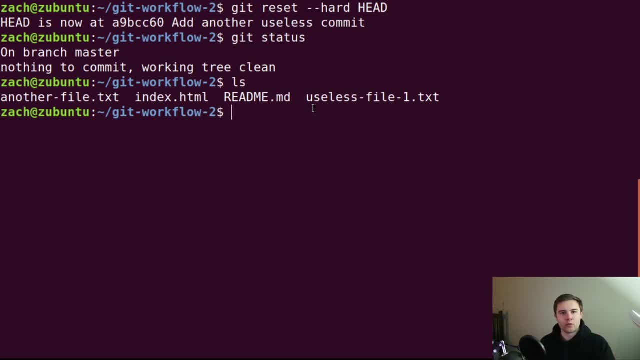 in your workflow, but again, be very careful with it, especially when using the hard flag on there, because it can essentially delete a bunch of work that you did. so that is the git reset command in a nutshell, and all three of those commands. the checkout revert. 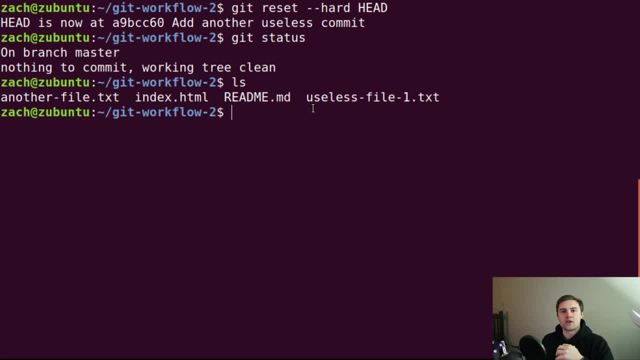 and reset commands. Hopefully you have a much better understanding of the differences between the three and have at least a general idea of when you might want to use them. so again, the git checkout command is when you want to just jump around in your repository. maybe you're switching branches to work on a different branch. 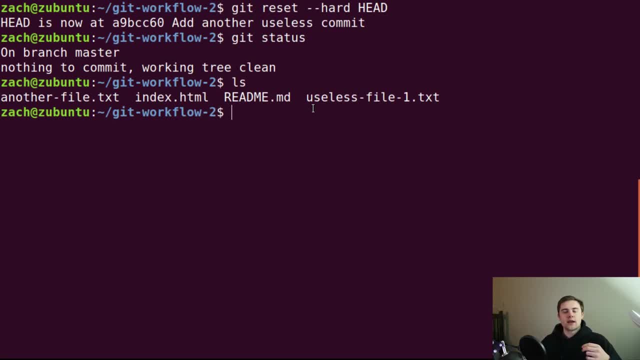 the revert command is if you want to kind of rewrite history without deleting anything in the history. so in other words, we go back to a snapshot and pull that forward in a new commit. so if we really wanted to, we could recover everything later. and then the reset command is: if you want to just 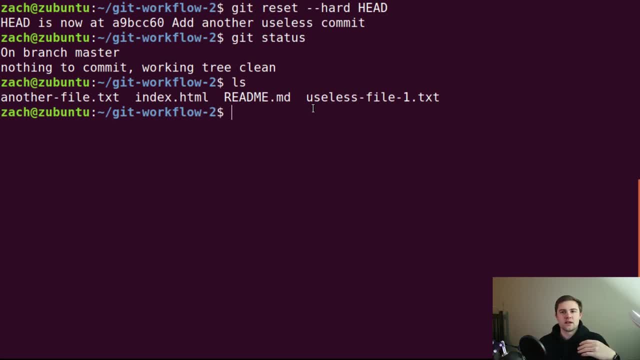 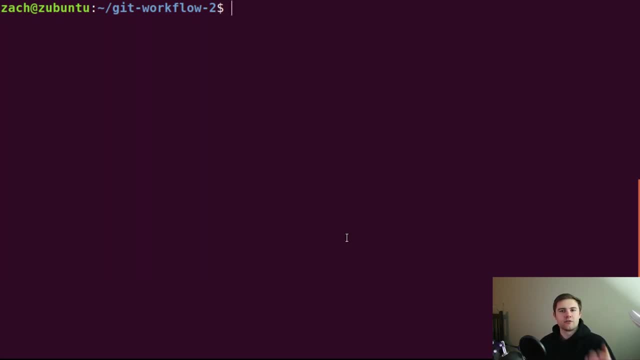 delete any commits. in general, you can delete commits with the git reset command. to bring this discussion kind of full circle, we had talked about merge conflicts at the beginning, especially with like pulling down from the remote repository to your local repository, but we never really talked about conflicts going the other way. 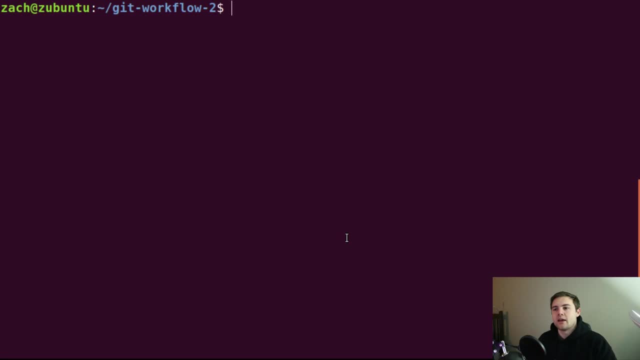 so if we want to push upstream and we have some changes locally that we want to throw into the repository, we didn't talk about those type of conflicts. in most cases you're not going to want to force anything when you're running the git push origin master command, but in our case we made 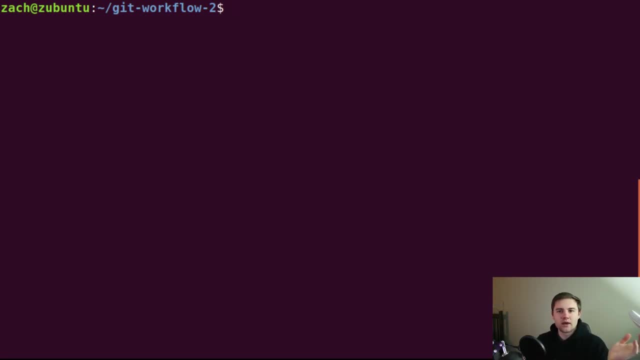 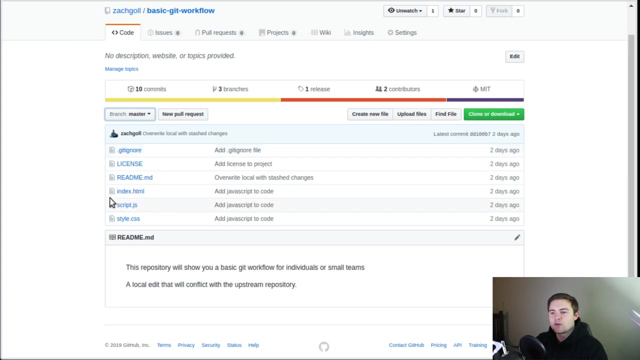 a bunch of changes. we went back in time, deleted some commits, added some commits and therefore the remote repository up on github has no idea what's going on. so if we go back to my github, if we look at this repository, we've got a bunch of files here on the master. 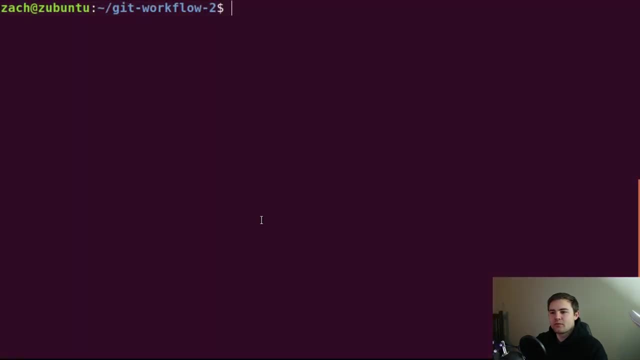 branch. but if we come back to our terminal you'll see that on the master branch we're on the master. right now we don't have anything that even resembles that. so maybe we wanted to take- for whatever reason we want to take- the files here and push those up to the remote repository. 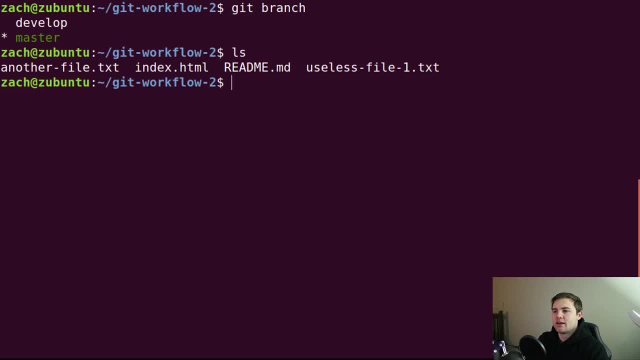 well, the only way that we'll be able to do that, and it's kind of a hacky way again. this will overwrite a remote repository and you need to use it with caution, especially if you're collaborating with others. but in our case, I'm just doing this alone and I know that the local 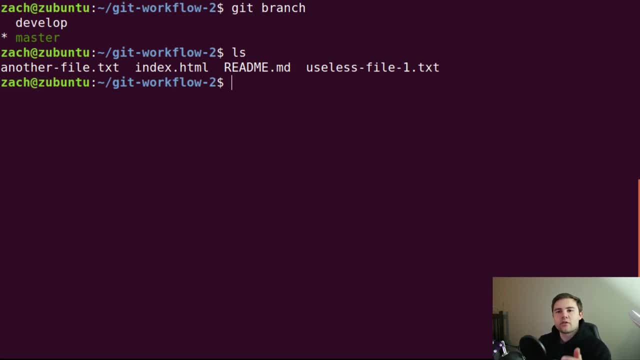 is the one that I want to throw up on github. so rather than you know, going on github deleting everything and recloning and just kind of resetting the entire thing, we can just type git push force. so this will force the local changes to overwrite the remote changes and then origin master. 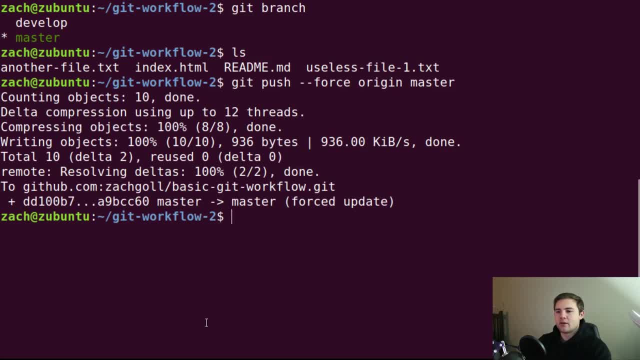 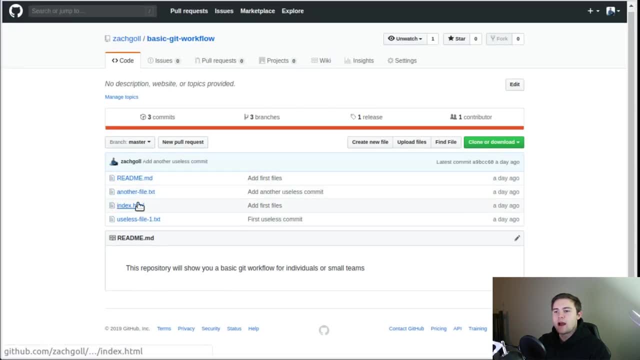 you'll see that we forced an update. and if we go back to the github and refresh, you'll see that we have all of these files and it now shows that there's only one contributor as opposed to two contributors before, so on and so forth. so that's how you.